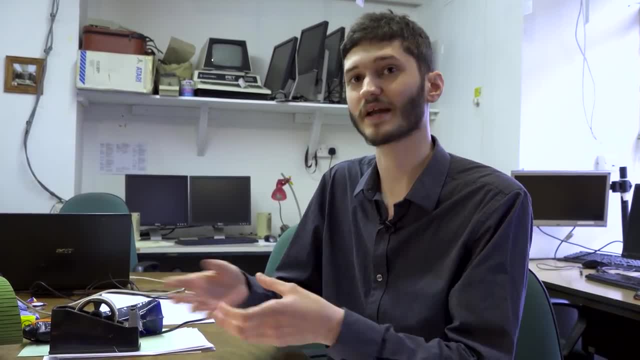 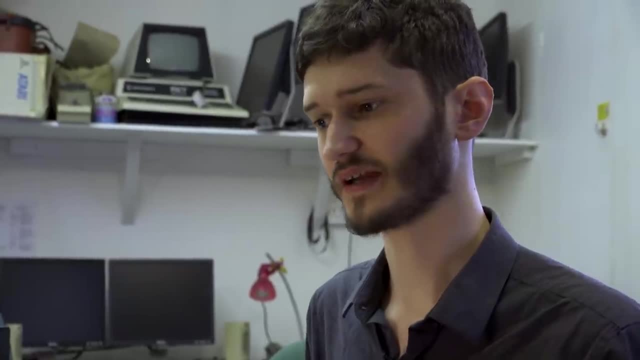 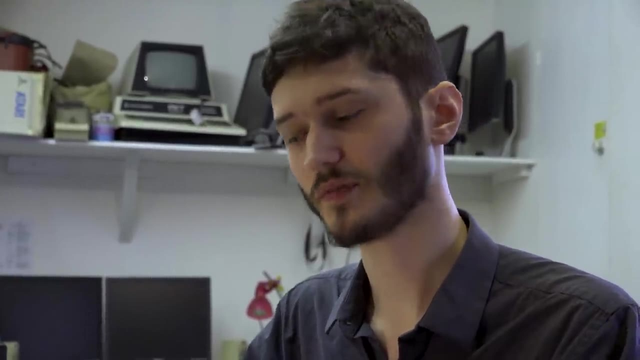 You can't say, okay, draw me a new cat picture, draw me a cat picture I haven't seen before. It doesn't know how to do that. So quite often you want a model that can generate new samples. So you give it a bunch of samples from a particular distribution and you want it to give you more samples which are also from that same distribution. 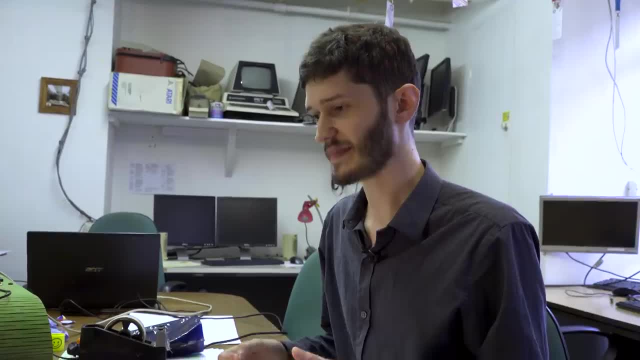 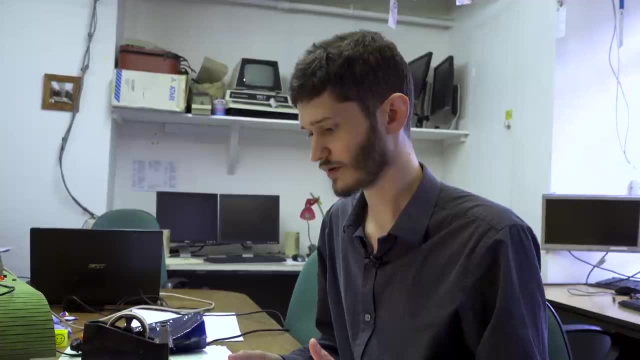 So it has to learn the underlying structure of what you've given it, And that's kind of tricky. actually, There's a lot of well, there's a lot of challenges involved in that. Well, to be honest, I think as a human, you can find that tricky. 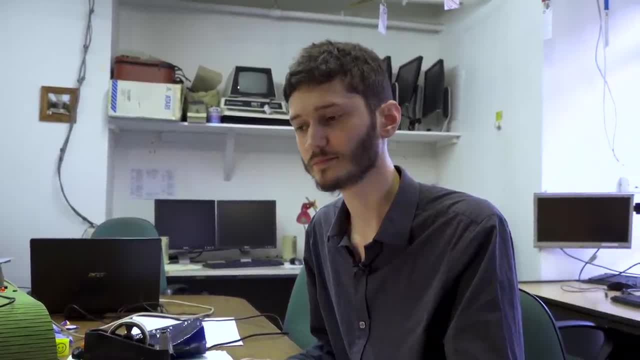 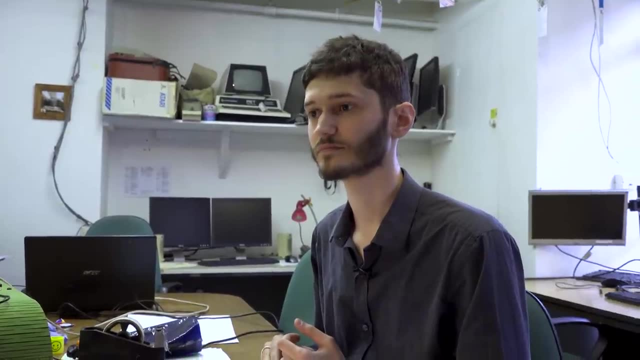 You know, if I know what a cat looks like, but being not the greatest artist in the world, I'm not sure that I could draw you a decent cat. So you know this is not confined to just computing, is it? 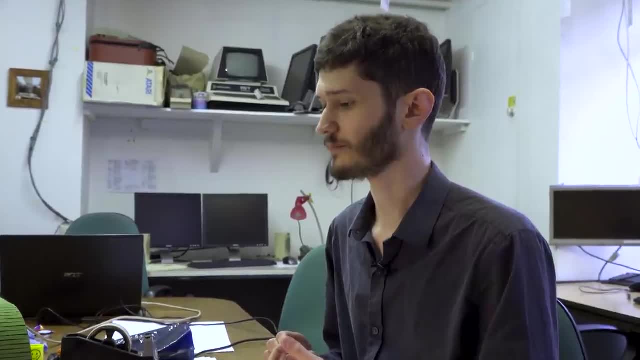 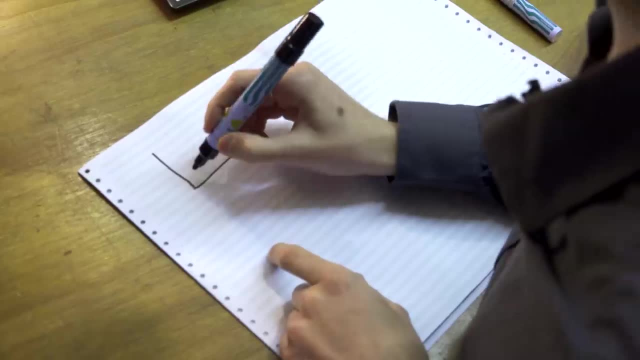 Yeah, that's true, That's really true. But if you take- let's do like- a really simple example of a generative model, Say, you give your network one thing, it looks like this, And then you give it another one. 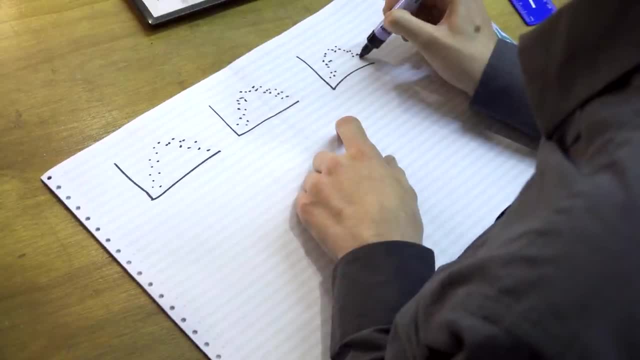 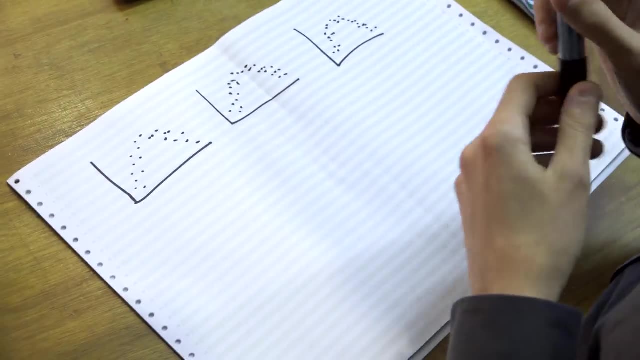 You're like: these are your training samples- Looks like this, And you give it another one that looks like this, And then What are those dots, in this instance, Instances of something on two dimensions? Yeah, I mean, right now it's literally just data. 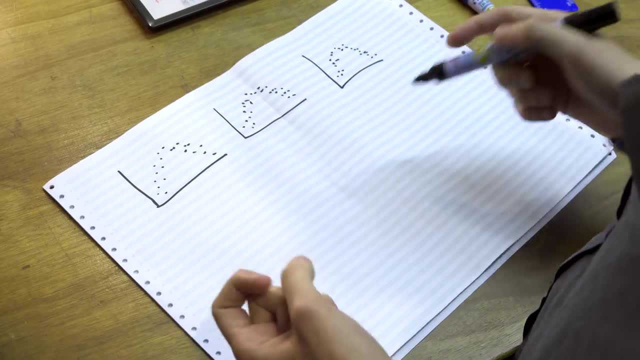 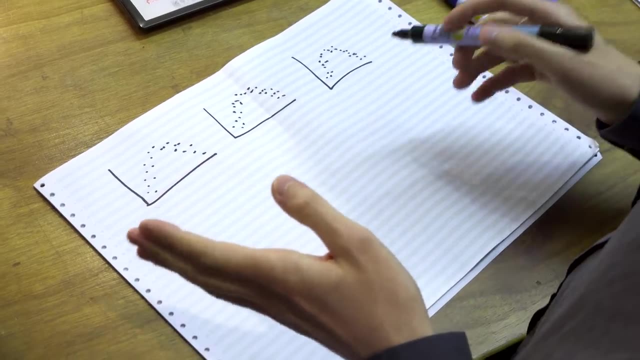 We're just: it doesn't matter what it is, Just some. yeah, these are data points, And so these are the things you're giving it, And then it will learn. you can train it. it will learn a model, And the model it might learn is something like this: 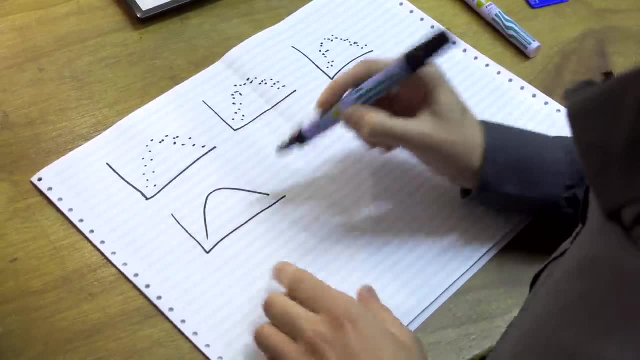 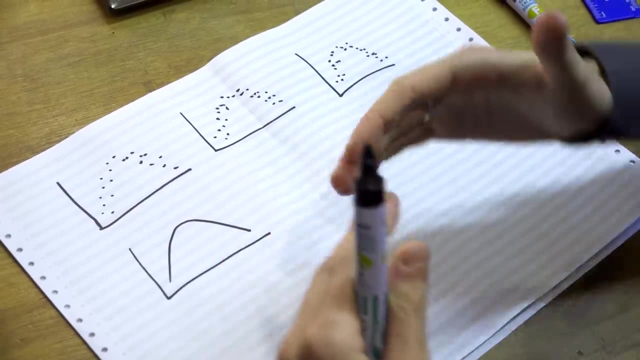 Right. It's figured out that these dots all lie along a path, And if its model was always to draw a line, then it could learn by adjusting the parameters of that line. It would move the line around until it found a line that was a good fit. 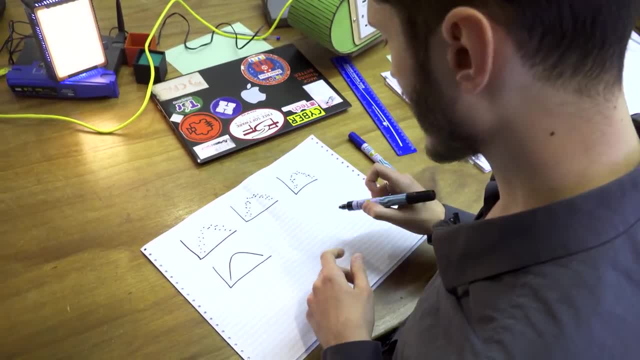 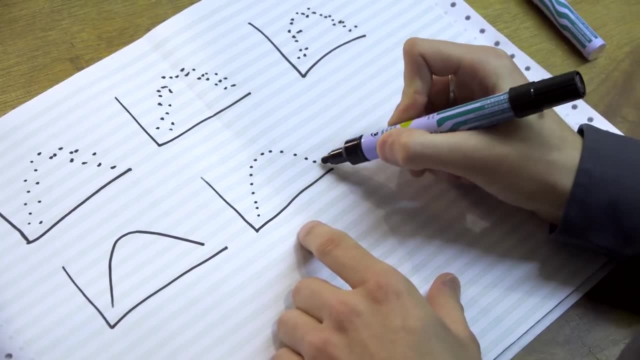 and generally gave you a good prediction. But then if you were to ask this model, okay, now make me a new one. Unless you did something clever, What you get is probably this: Because that is, on average, the closest to any of these. 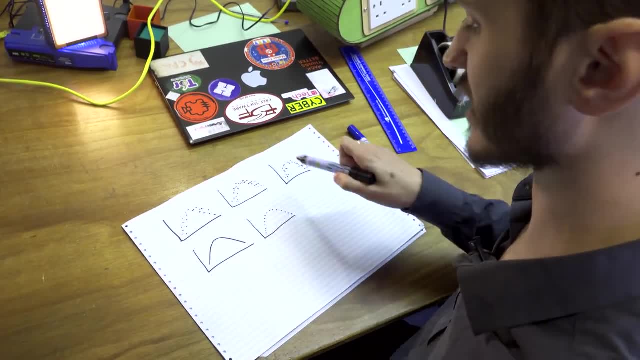 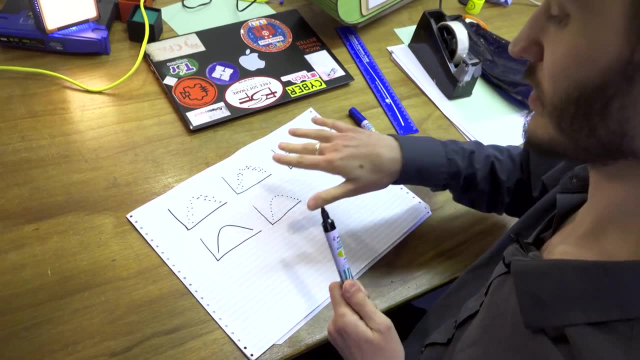 Because any of these dots- you don't know if they're going to be above or below, or you know, to the left or the right- There's no pattern there. It's kind of random. So the best place you can go, that will minimize your error. 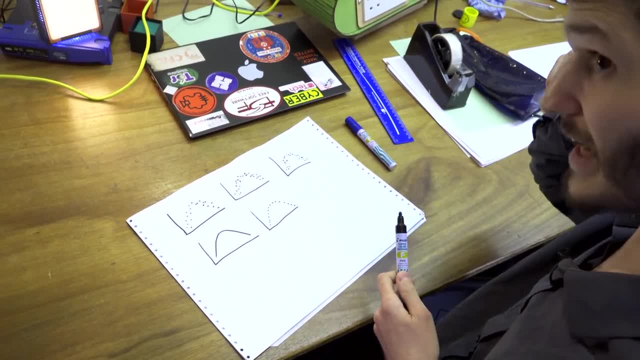 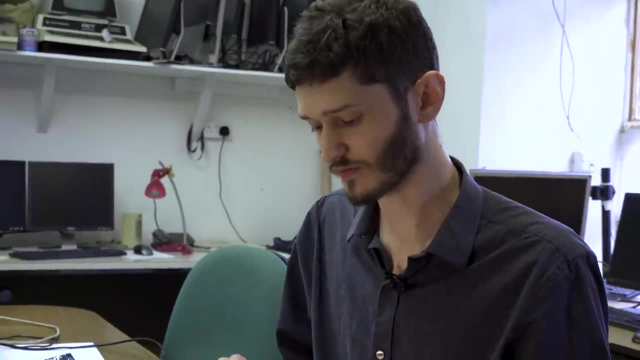 is to go just right on the line every time. But anybody looking at this will say, well, that's fake. That's not a plausible example of something from this distribution, even though for a lot of the like error functions that people use. 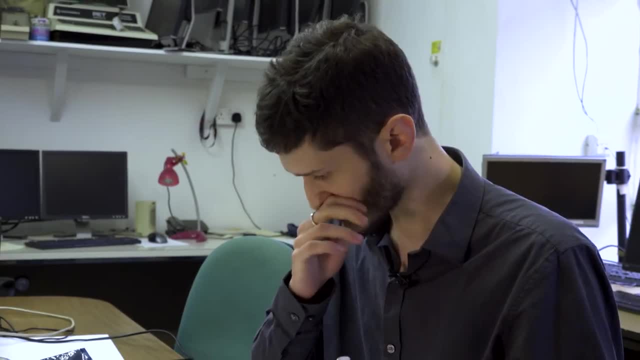 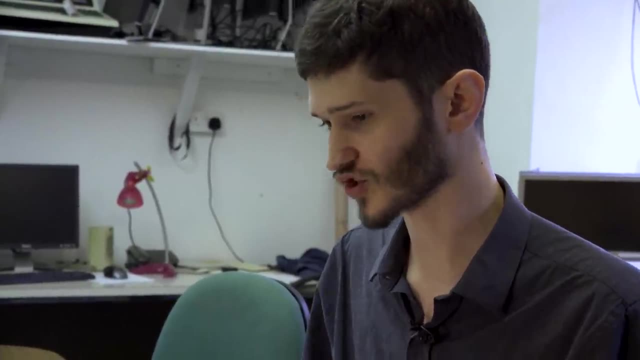 when training networks, this would perform best. So it's this interesting situation where there's not just one right answer. You know, generally speaking, the way that neural networks work is you're training them towards a specific, you have a label or you have an output, a target output. 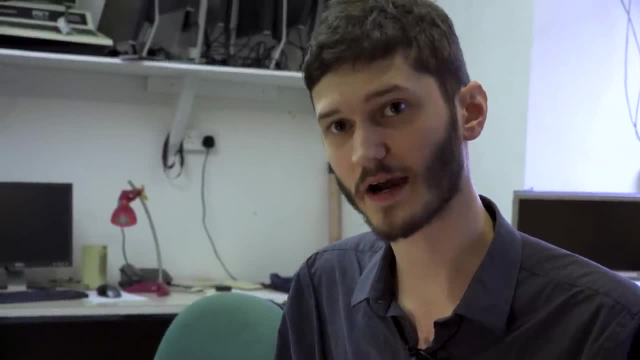 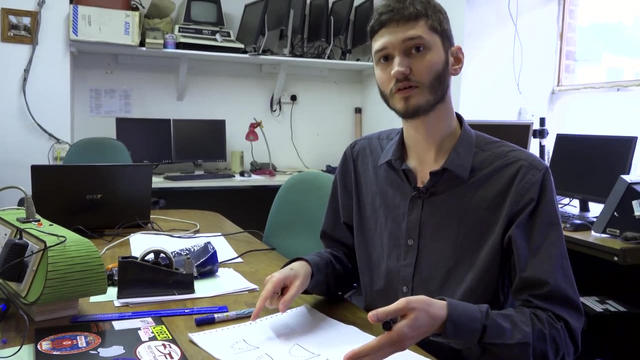 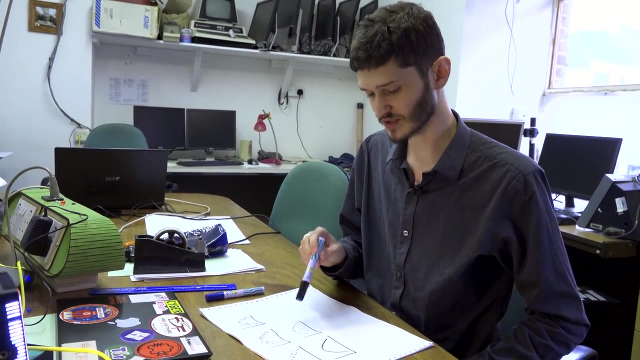 and you get penalty the further away you are from that output, Whereas in an application like this, there's basically an infinite number of perfectly valid outputs here. So to generate this, what you'd actually need is to take this model and then apply some randomness. 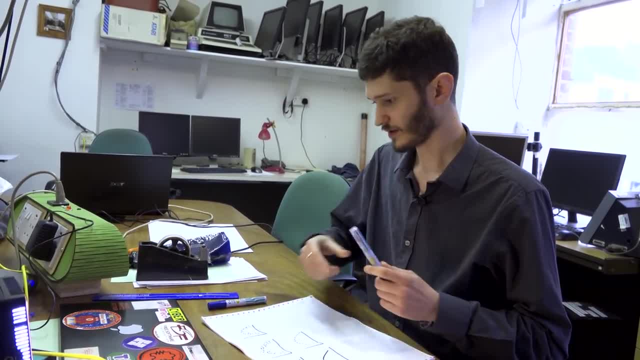 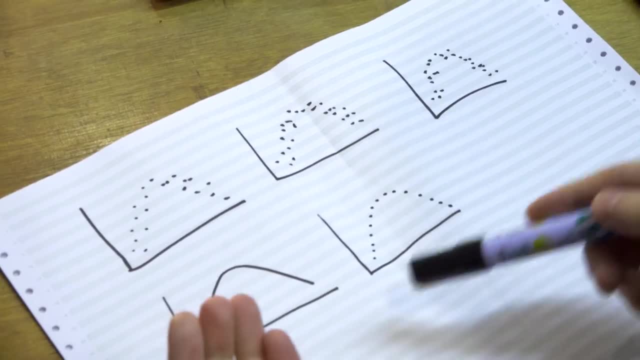 You say they're all within. you know they occur randomly and they're normally distributed around this line with this standard deviation or whatever. But a lot of models would have a hard time actually picking one of all of the possibilities and they would have this tendency. 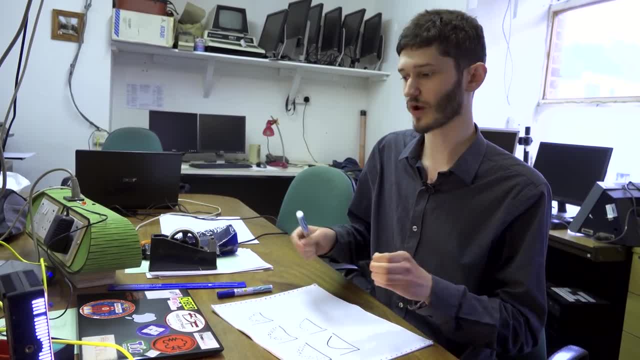 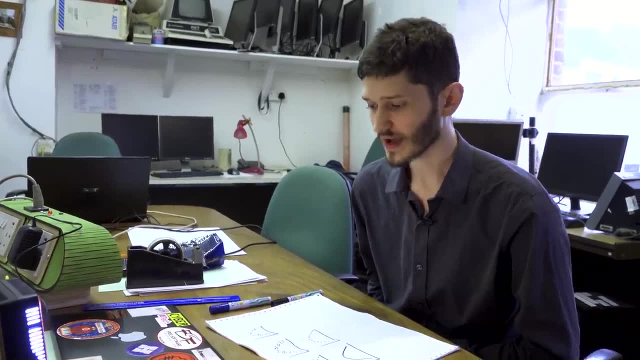 to kind of smooth things out and go for the average, whereas we actually just want just pick me one, It doesn't matter. So that's part of the problem of generating Adversarial training is a lot of work. It's a way of training, not just networks actually, 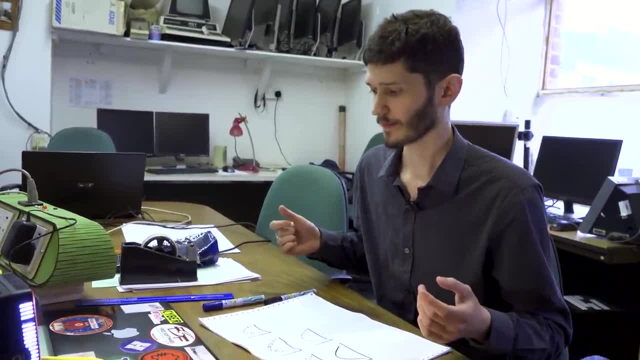 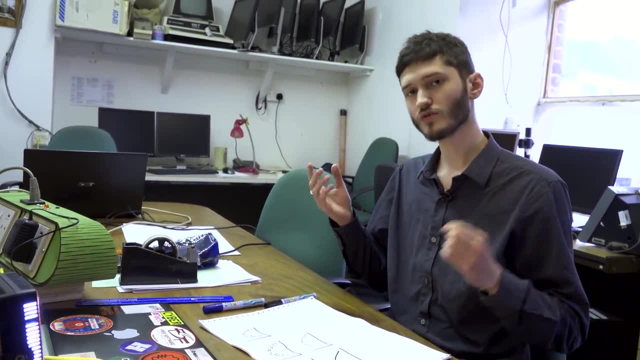 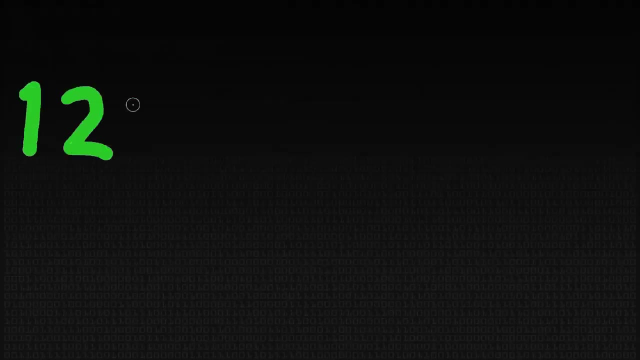 a way of training machine learning systems, which involves focusing on the system's weaknesses. So if you are learning- let's say you're teaching your network to recognize handwritten digits the normal way you would do that- you have your big training sample of labeled samples. 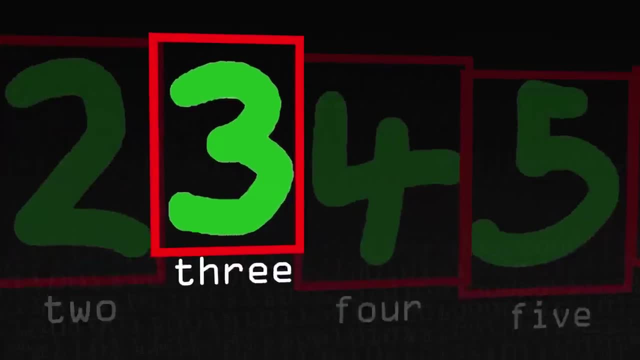 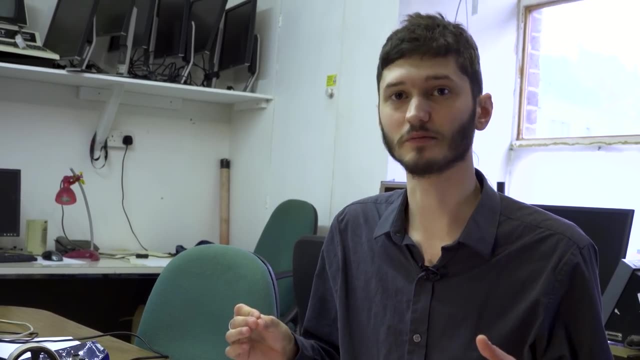 You've got an array of pixels that looks like a three and then it's labeled with three and so on, And the normal way that you would train a network with this is you would just present all of them pretty much at random. You'd present as many ones as twos as threes. 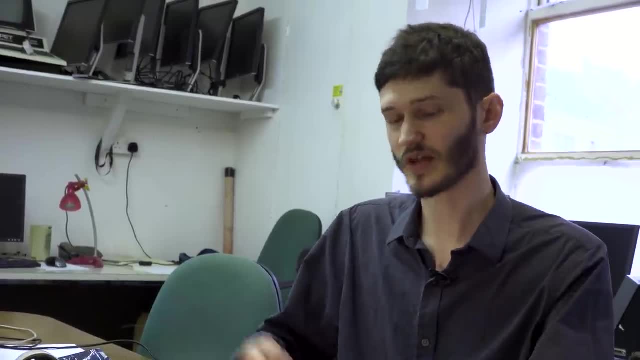 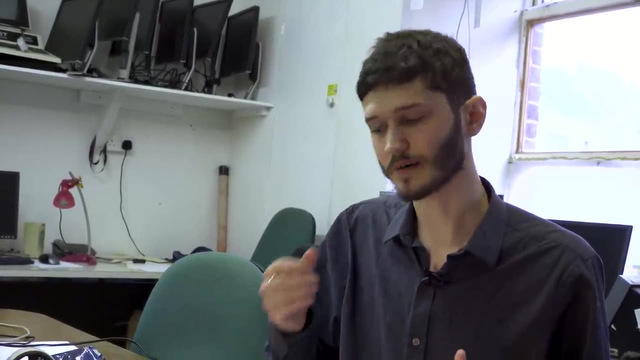 and just keep throwing examples at it. What's this? You know? yes, you got that right. No, you got that wrong. It should really be this And keep doing that and the system will eventually learn. But if you were actually teaching a person to recognize the numbers, 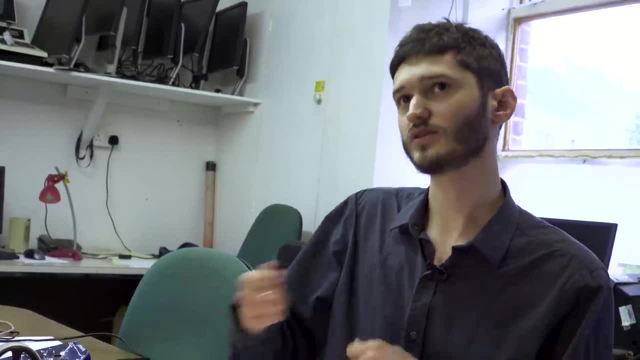 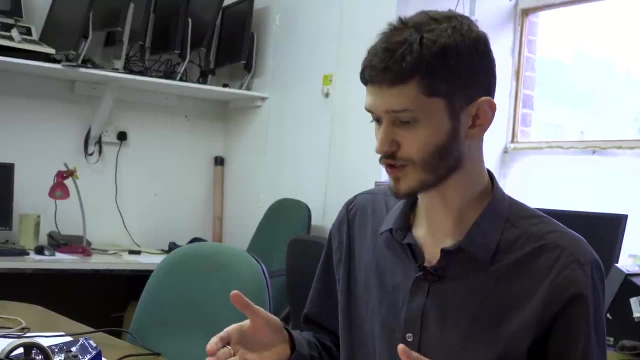 if you were teaching a child, you wouldn't do that, Like if you'd been teaching them for a while, presenting them and getting the response and correcting them and so on, and you noticed that they can do with two, three, four, five, six, eight and nine. 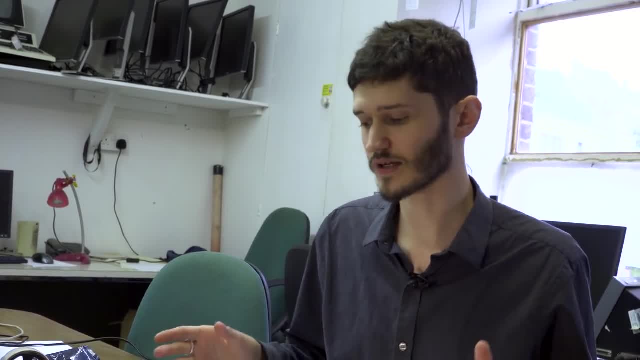 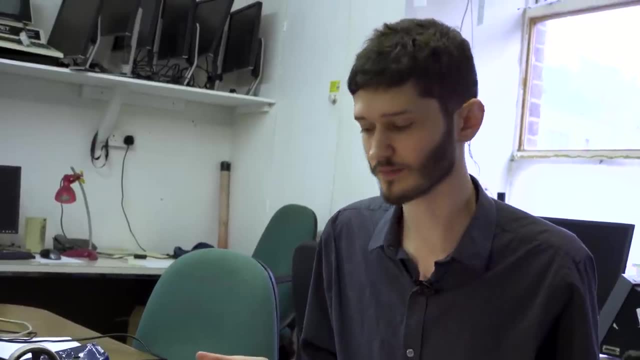 they're getting like 70%, 80% accuracy recognition rate, but one and seven it's like 50-50 because they keep any time they get a one or a seven. they just guess because they can't tell the difference between them. 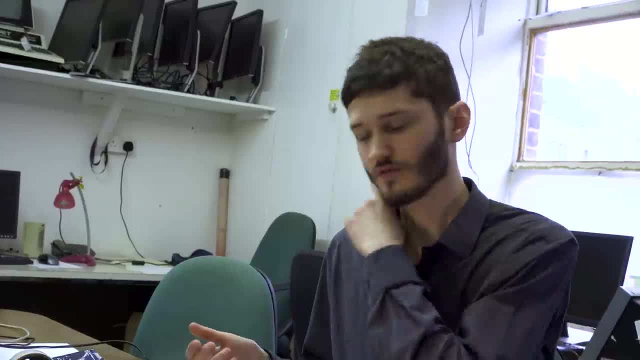 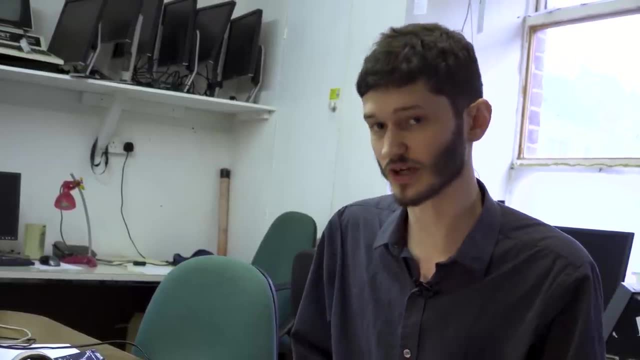 If you noticed that you wouldn't keep training those other numbers, You would stop and say: well, you know what. We're just going to focus on one and seven, because this is an issue for you, I'm going to keep showing you ones and sevens and correcting you. 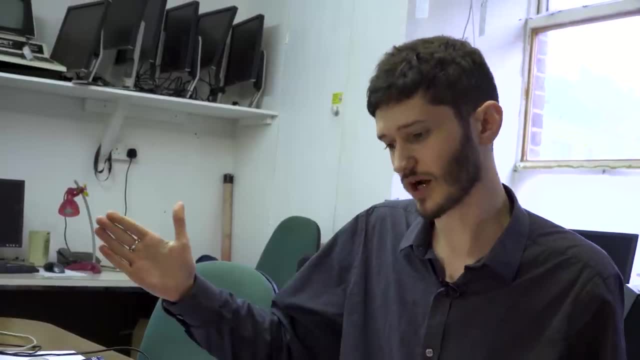 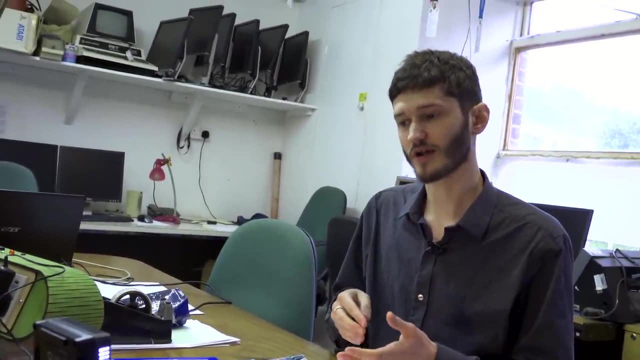 until the error rate on ones and sevens comes down to the error rate that you're getting on your other numbers. You're focusing the training on the area where the student is failing And there's kind of a balance there when you're teaching humans. 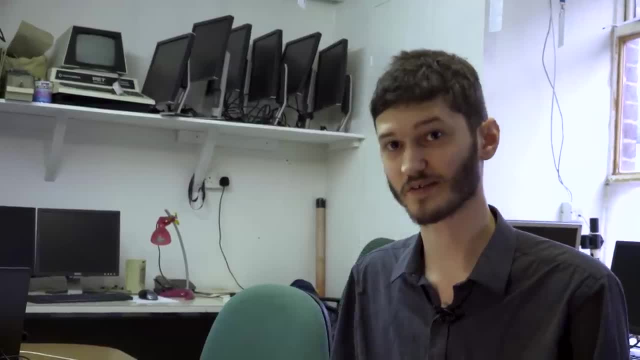 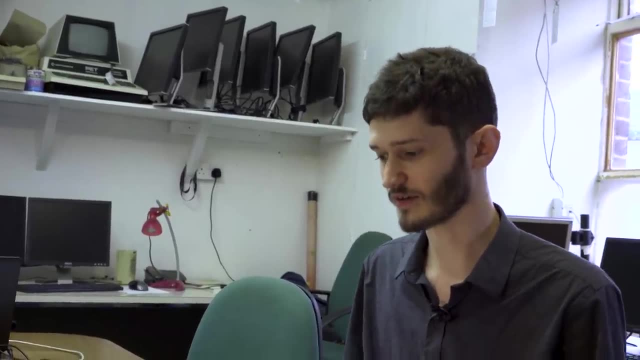 because if you keep relentlessly focusing on their weaknesses and making them do stuff they can't do, all the time they will just become super discouraged and give up. But neural networks don't have feelings yet, so that's really not an issue. You can just continually hammer on the weak points. 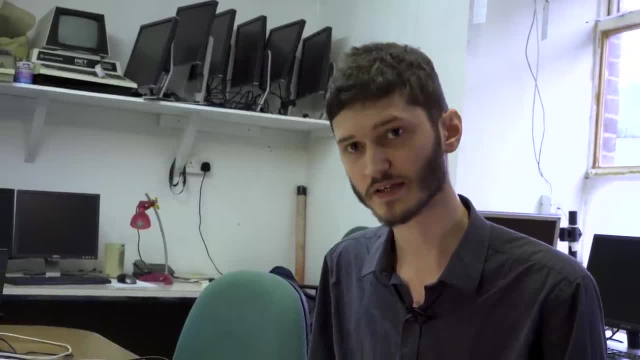 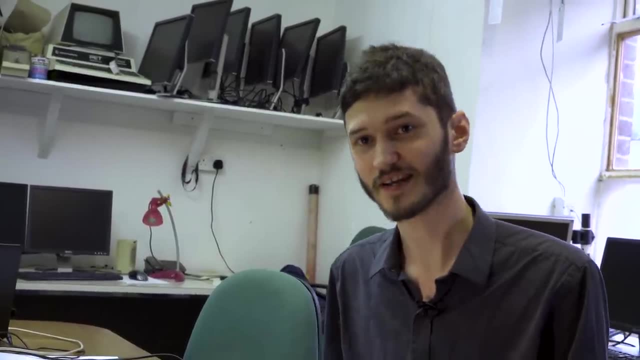 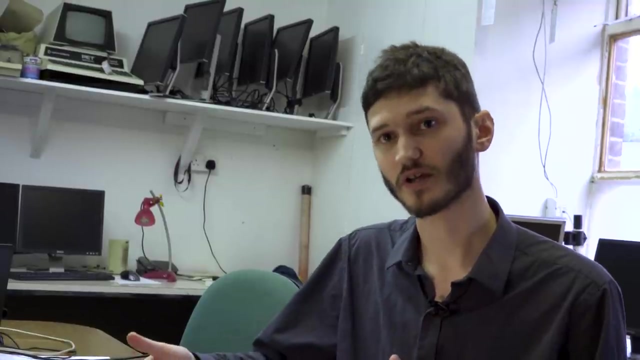 find whatever they're having trouble with and focus on that. And so that behavior- and I think some people have had teachers where it feels like this, it feels like an adversary right, It feels like they want you to fail, So in fact, you can make them an actual adversary- 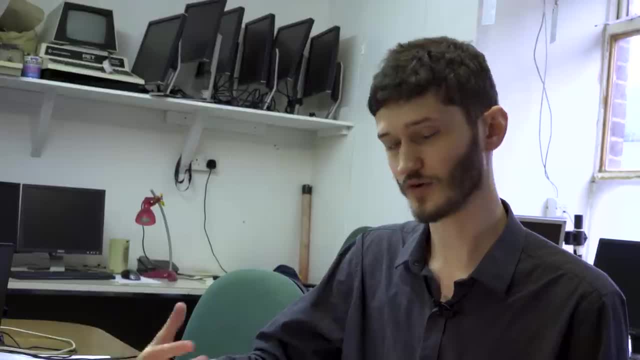 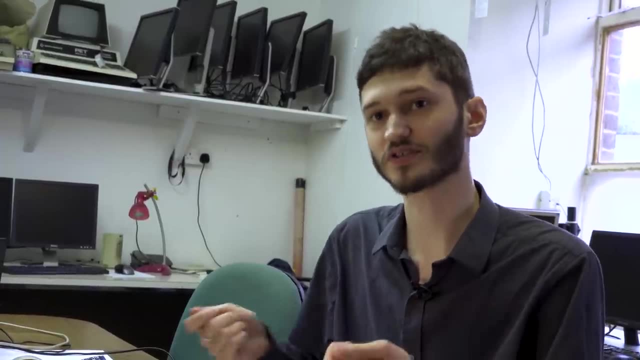 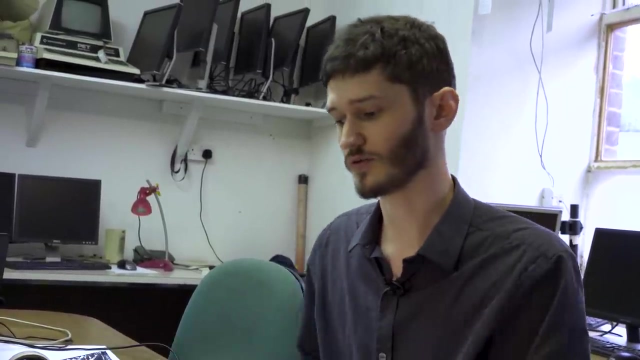 if you have some process which is genuinely doing its best to make the network give as high an error as possible, That will produce this effect where, if it spots any weakness, it will focus on that and thereby force the learner to learn to not have that weakness anymore. 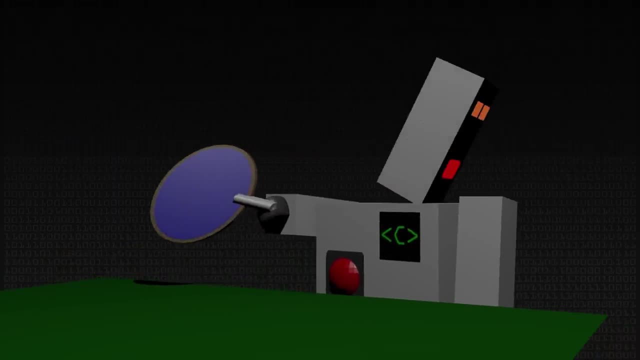 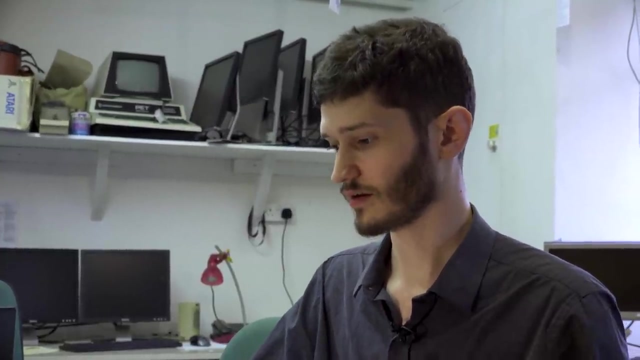 Like one form of adversarial training people sometimes do is if you have a game-playing program, you make it play itself a lot of times, because all the time they are trying to look for weaknesses in their opponent and exploit those weaknesses, And when they do that they're forced to then improve. 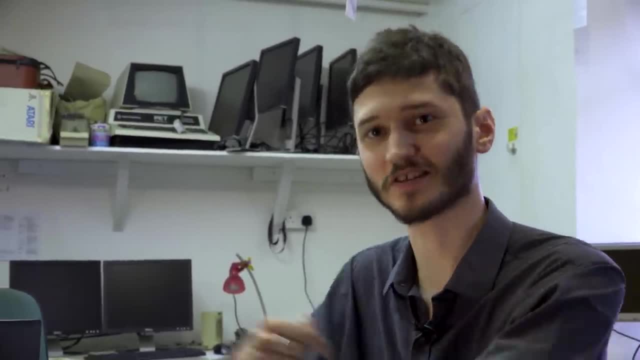 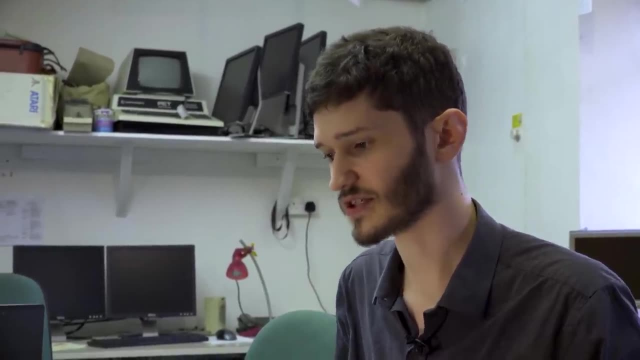 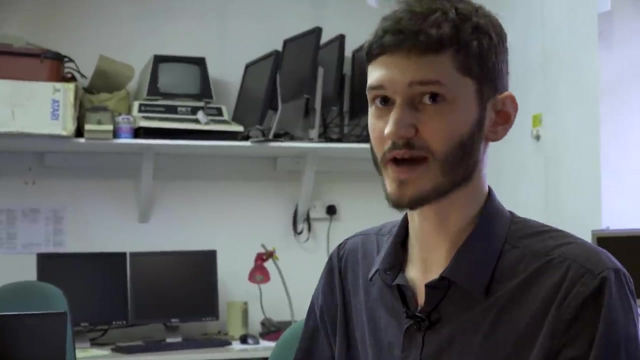 or fix those weaknesses in themselves, because their opponent is exploiting those weaknesses. So every time the system finds a strategy that is extremely good against this opponent, the opponent who's also them has to learn a way of dealing with that strategy, and so on, and so on. 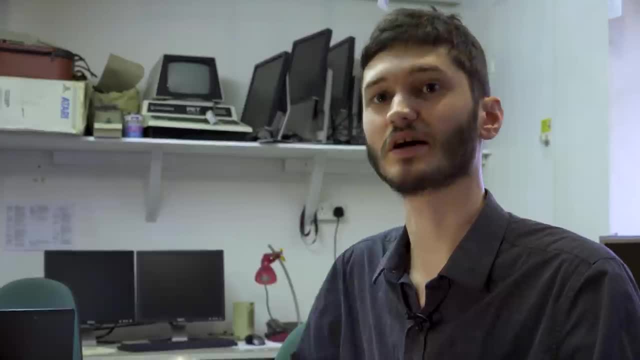 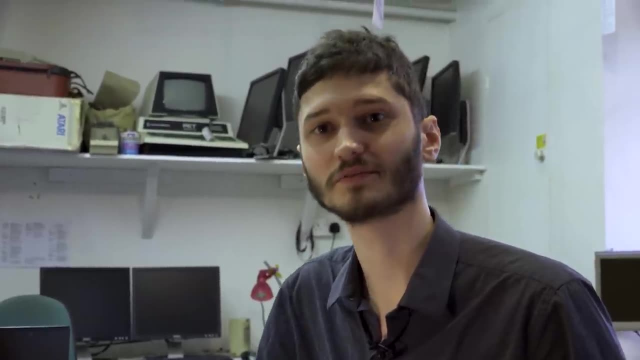 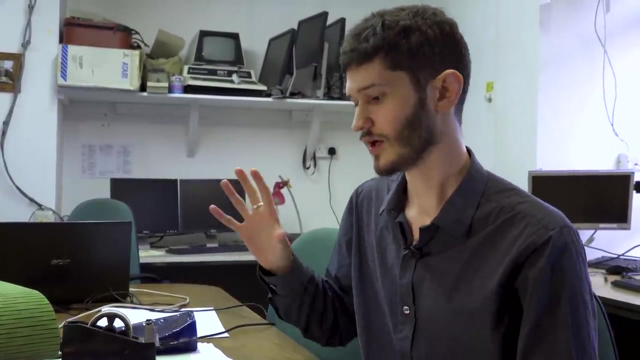 So as the system gets better, it forces itself to get better because it's continuously having to learn how to play a better and better opponent. It's quite elegant, you know. This is where we get to generative adversarial networks. Let's say: you've got a network. 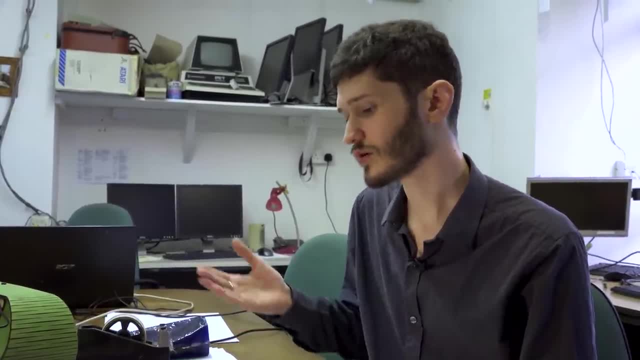 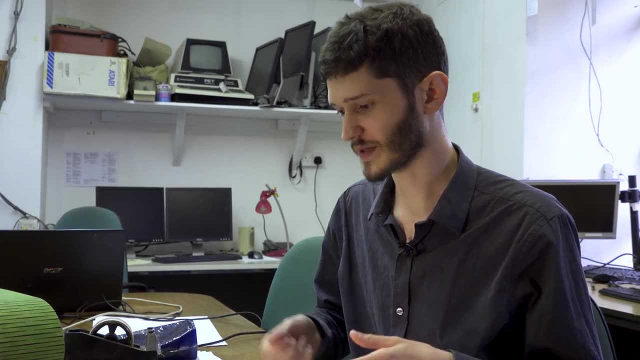 You want to. Let's say you want cat pictures. you know You want to be able to give it a bunch of pictures of cats and have it spit out a new picture of a cat that you've never seen before. That looks exactly like a cat. 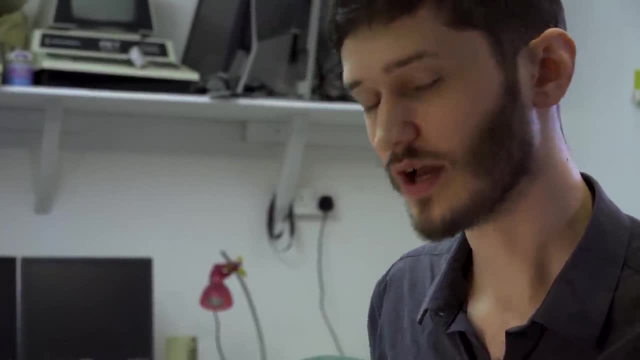 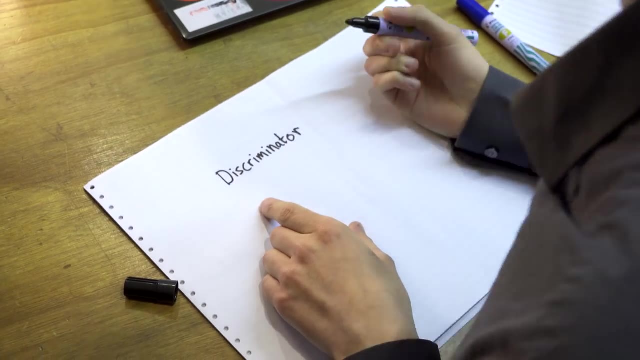 The way that a generative, adversarial network works is it's this architecture, where you actually have two networks. One of the networks is the discriminator. Ooh, how's my spelling? Yeah, I like that. The discriminator network is a classifier right. 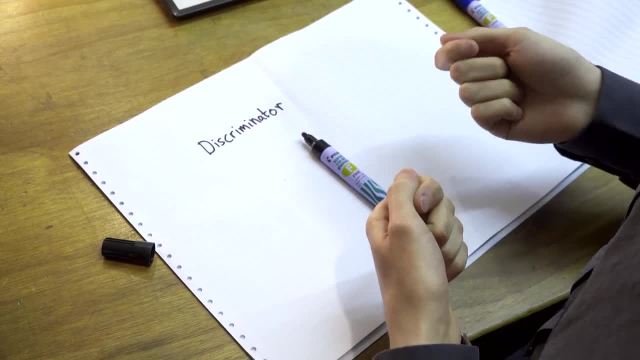 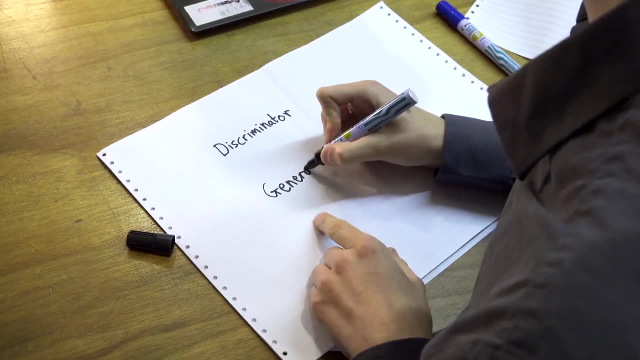 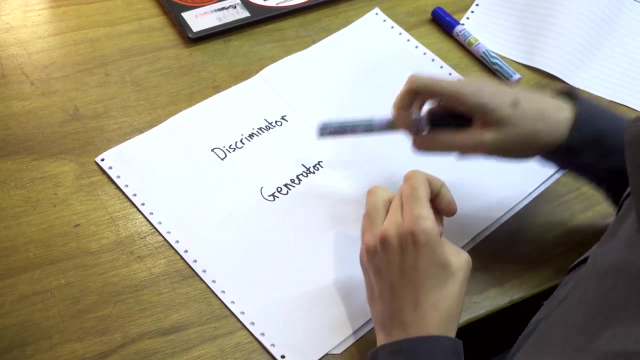 It's a straightforward classifier. You give it an image and it outputs a number between 0 and 1. And you're training that in standard supervised learning way. Then you have a generator, And the generator is usually a convolutional neural network. 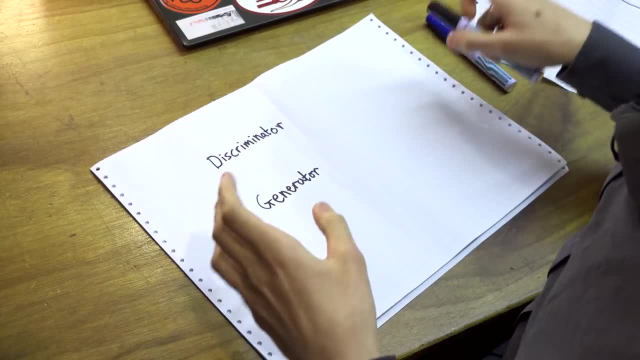 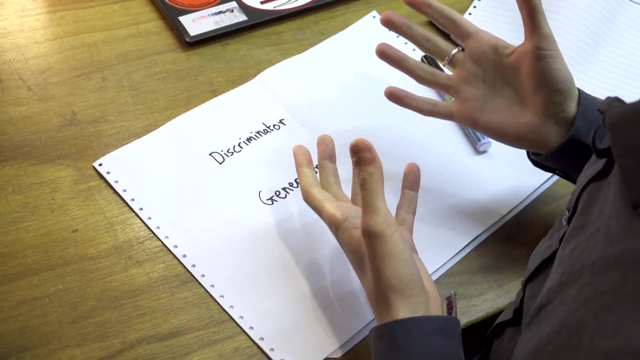 although actually both of these can be other processes, but people tend to use neural networks for this- And the generator. you give it some random noise and that's where it gets its source of randomness, so that it can give multiple answers to the same question effectively. 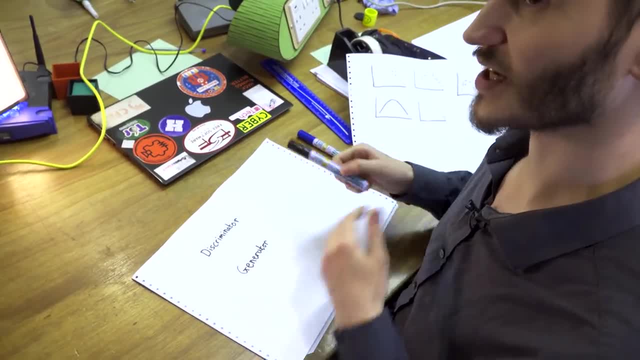 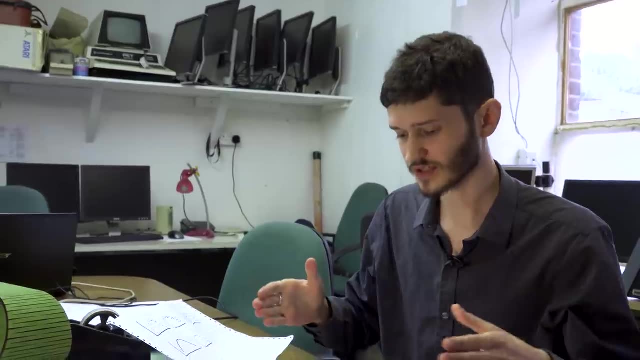 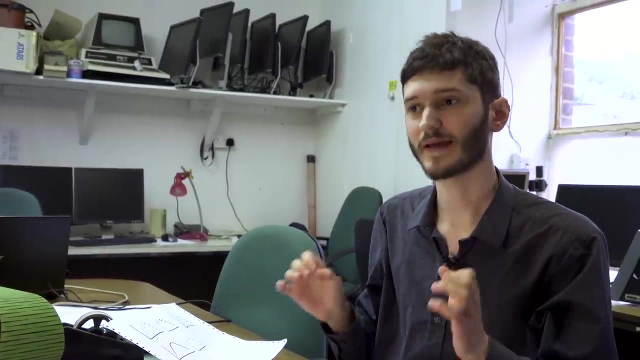 You give it some random noise and it generates an image from that noise and the idea is it's supposed to look like a cat. So the way that we do this with a generative adversarial network is it's this architecture whereby you have two networks playing a game effectively. 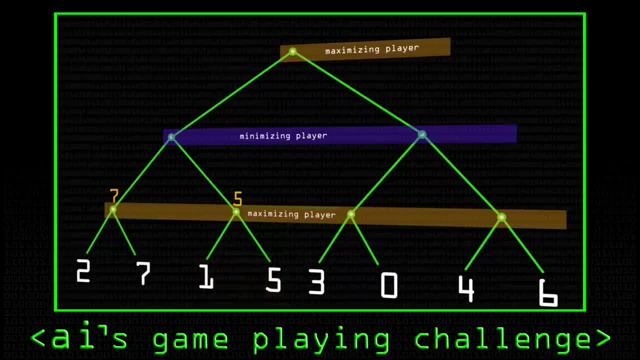 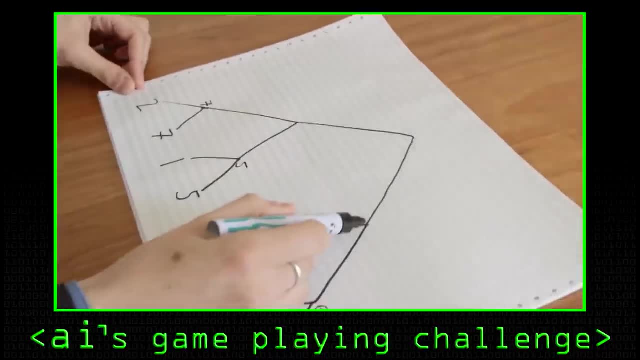 It's a competitive game, It's adversarial between them And in fact it's a very similar kind of game to the games we talked about in the previous AlphaGo video right. It's a min-max game because these two networks are fighting over one number. 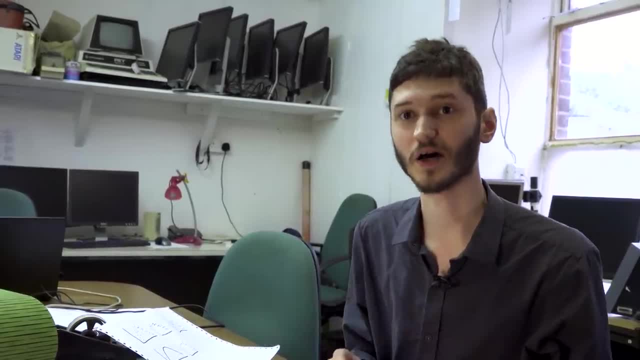 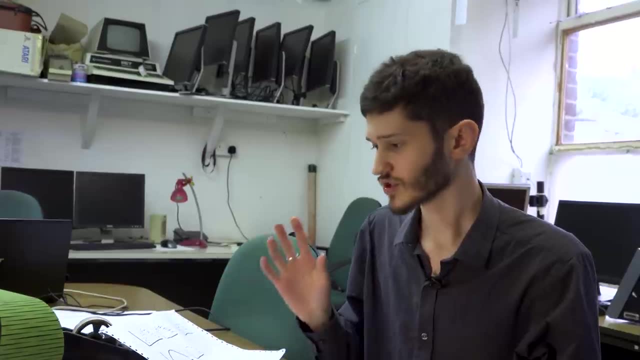 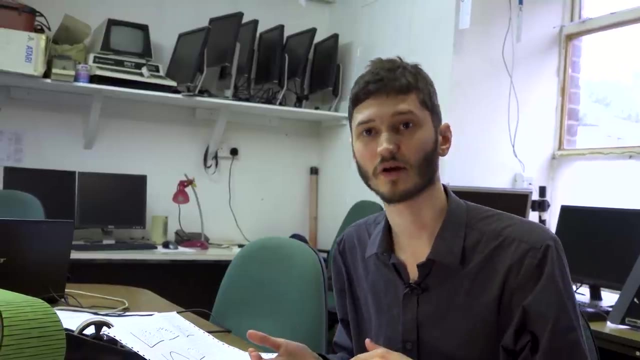 One of them wants the number to be high. One of them wants the number to be low, And what that number actually is is the error rate of the discriminator. So the discriminator wants a low error rate. The generator wants a high error rate. 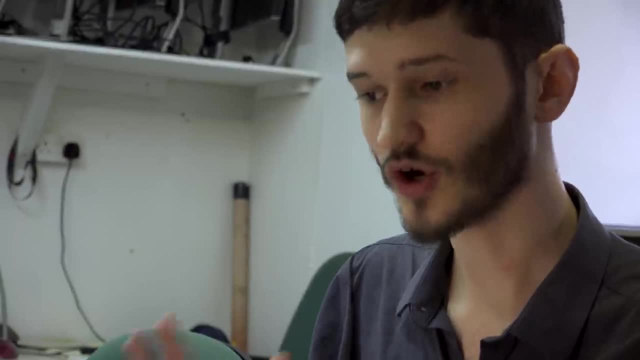 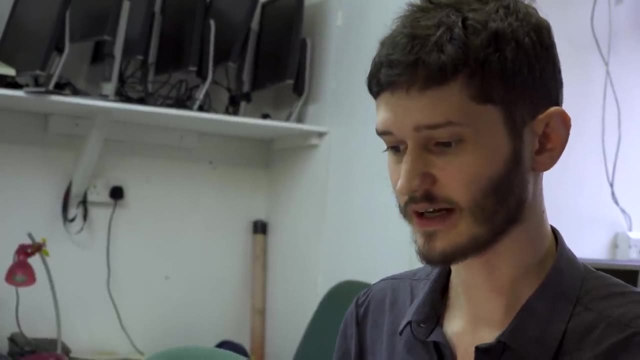 The discriminator's job is to look at an image which could have come from the original data set or it could have come from the generator, and its job is to say, yes, this is a real image or no, this is fake, And it outputs a number between 0 and 1,. 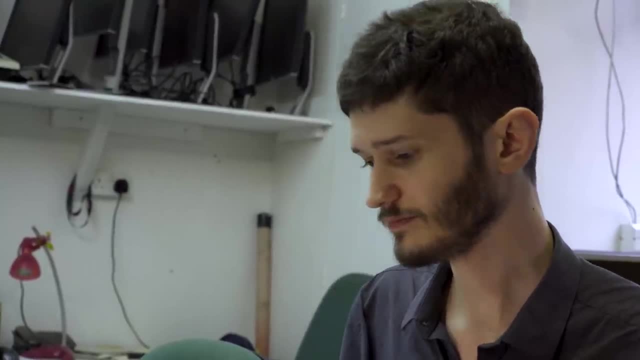 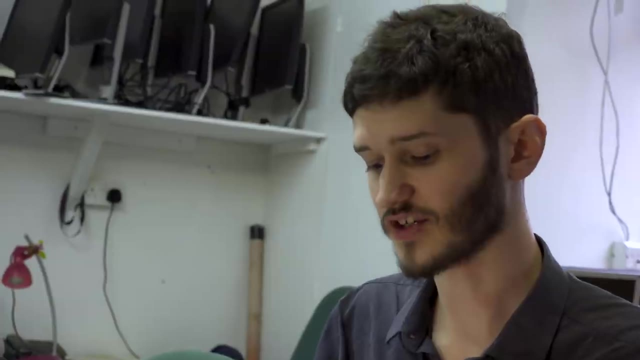 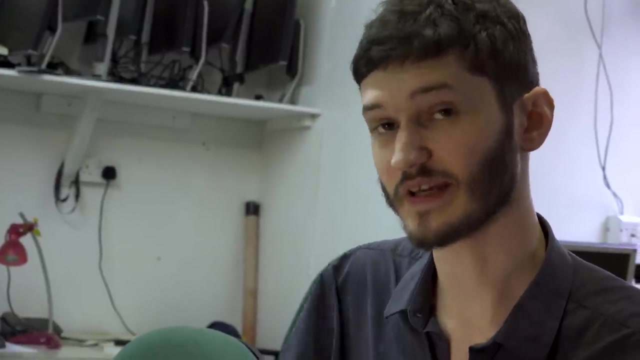 like 1 for it's real and 0 for it's fake, for example, And the generator gets fed as its input just some random noise And it then generates an image from that, And its reward, its training, is pretty much the inverse. 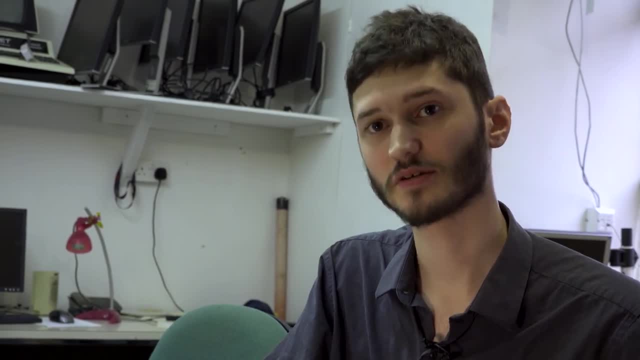 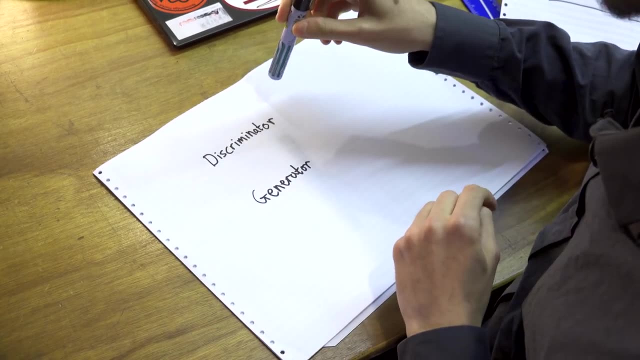 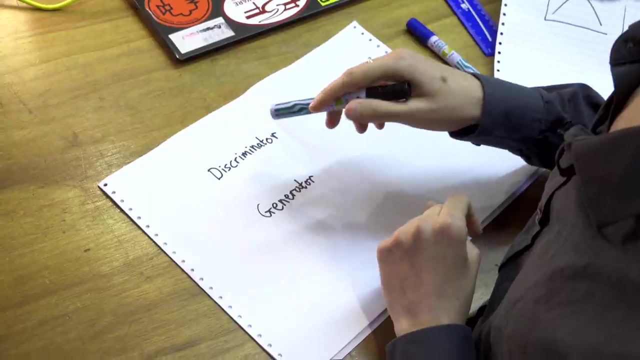 of what the discriminator says for that image. So if it produces an image which the discriminator can immediately tell is fake, it gets a negative reward. It's trained not to do that If it manages to produce an image that the discriminator can't tell is fake. 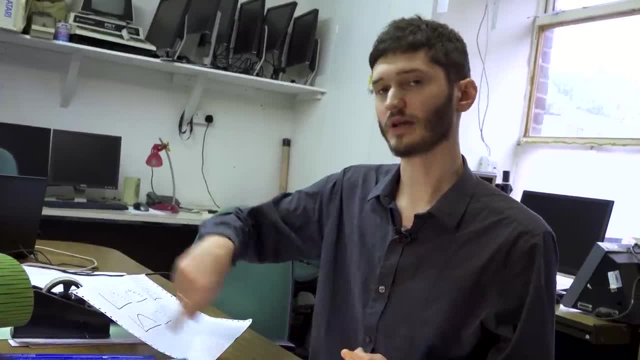 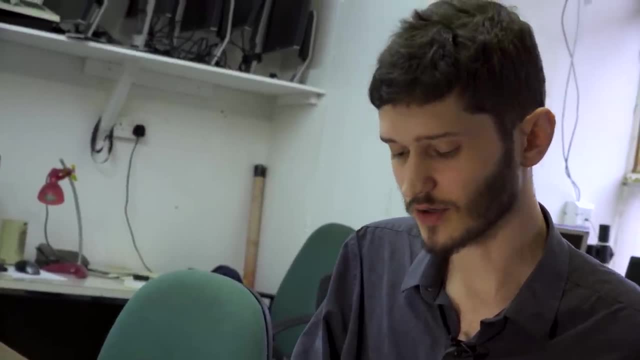 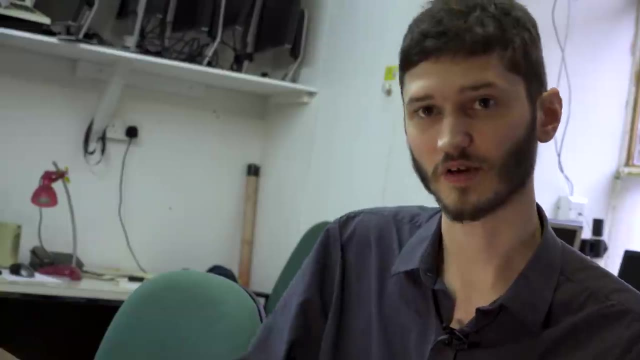 then that's really good. So you train them in a cycle effectively. You give the discriminator a real image, get its output. Then you generate a fake image and give the discriminator that And then you give it a real. So the discriminator gets alternating: real image, fake image, real image, fake image. 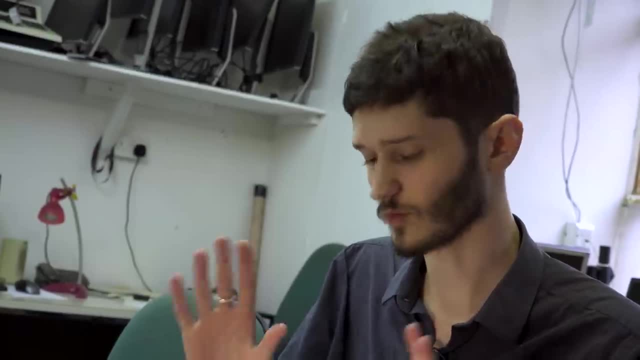 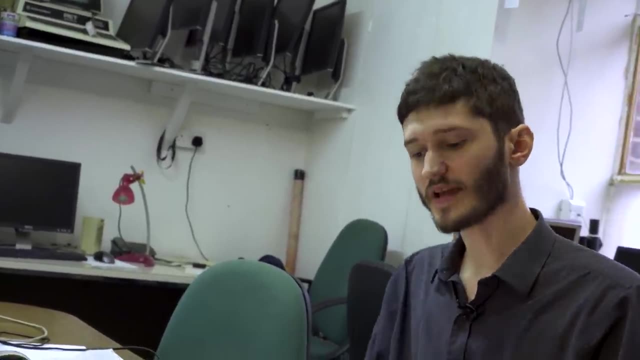 Usually. I mean, there are things you can do where you train them at different rates and whatever, But by default, Does the generator get any help with this at all, or is it purely Yes? So if you, This is like part of what makes this especially clever, actually. 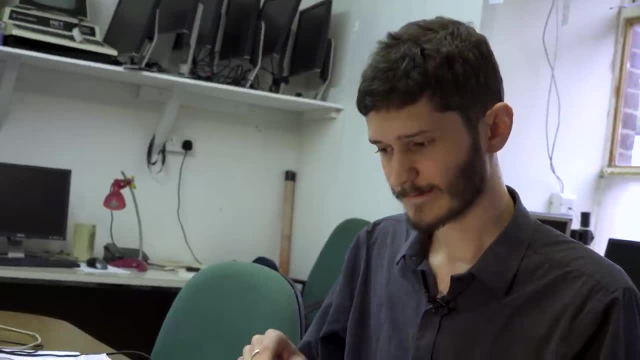 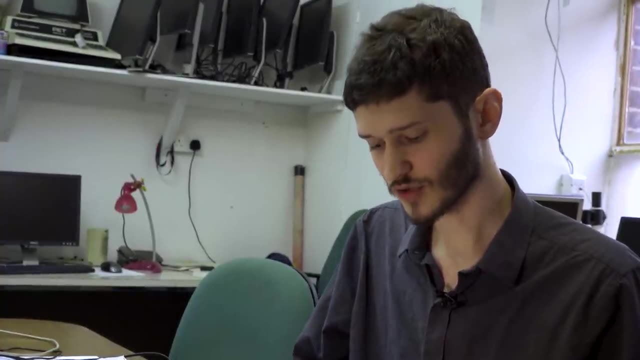 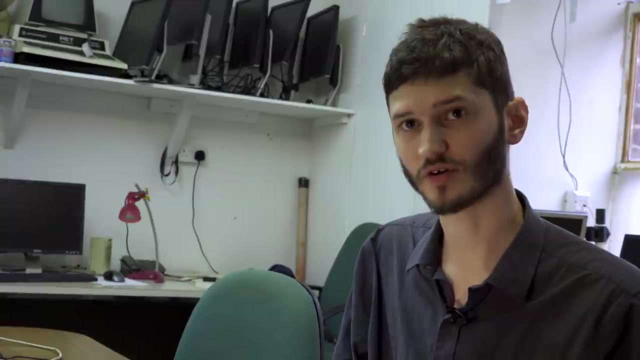 The generator does get help because if you set up the networks right you can use the gradient of the discriminator to train the generator. So when I know you've done back propagation before about how neural networks are trained, It's gradient descent right. 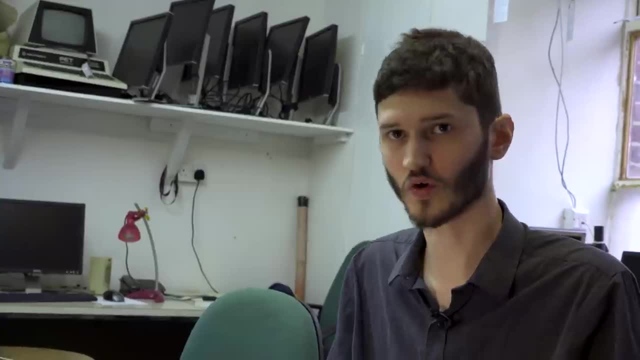 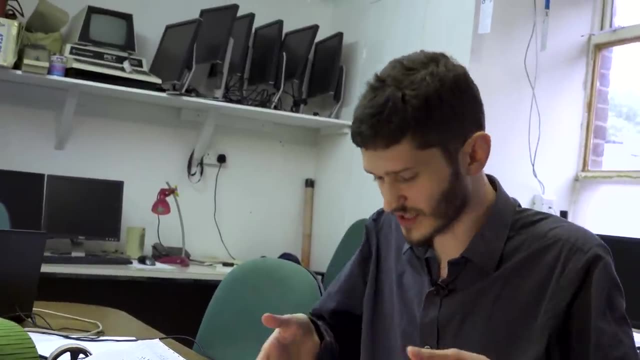 And in fact, we talked about this in like 2014.. If you're a blind person climbing a mountain or it's really foggy and you're climbing a mountain, you can only see directly what's underneath your own feet. You can still climb that mountain if you just follow the gradient. 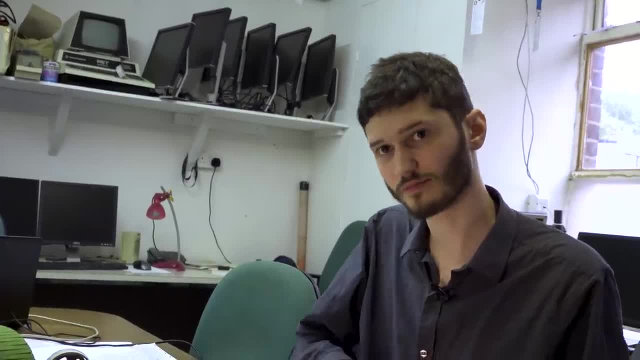 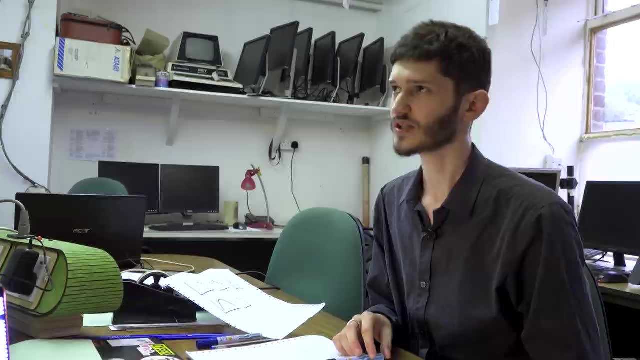 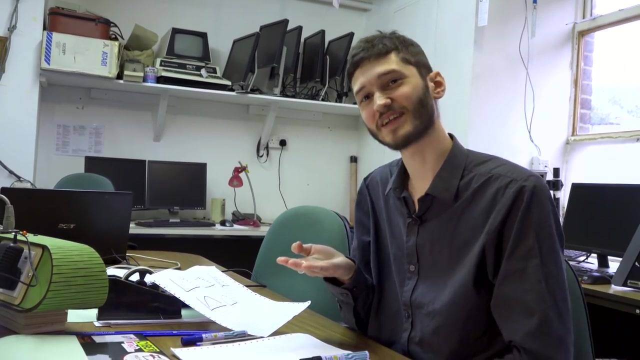 You just look directly under me. which way is the ground sloping? This is when we did the hill climb algorithm, Exactly. Yeah, Sometimes people call it hill climbing, Sometimes people call it gradient descent. It's the same metaphor upside down, effectively, if we're climbing up or we're climbing down. 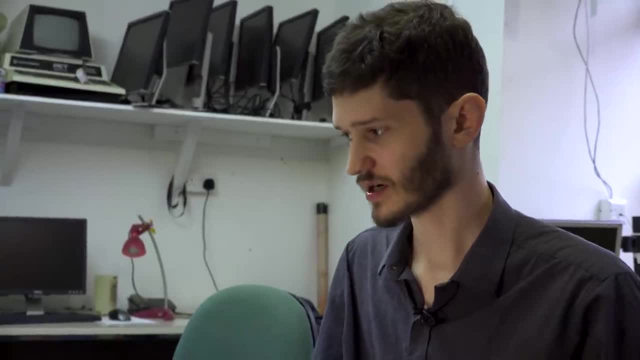 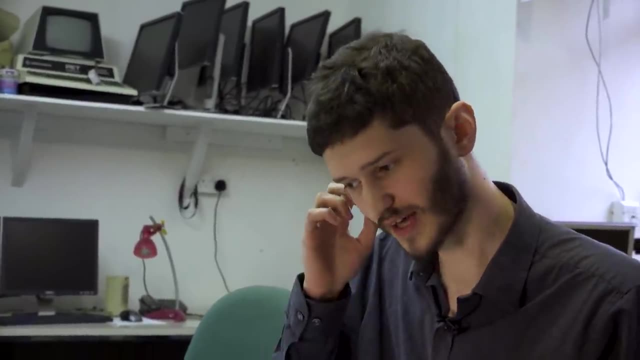 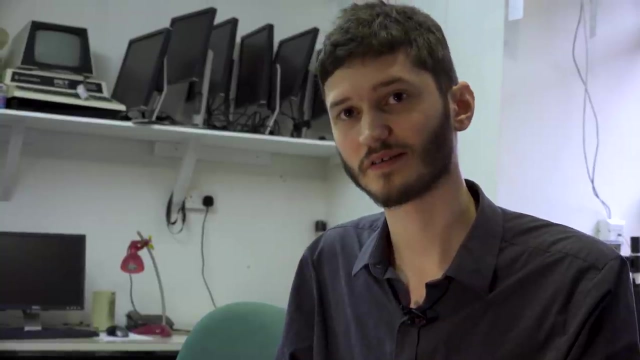 You're training them by gradient descent, which means that you're not just able to say, yes, that's good, no, that's bad. You're actually able to say, and you should adjust your weights in this direction so that you'll move down the gradient right. 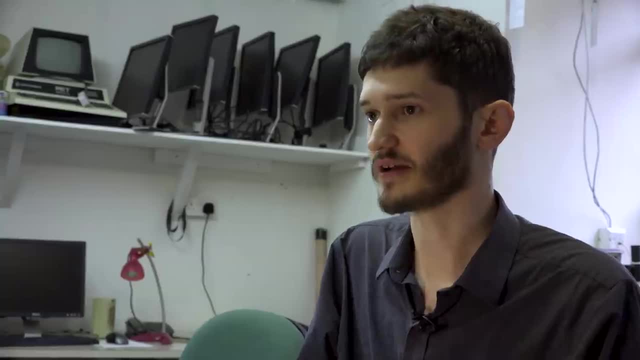 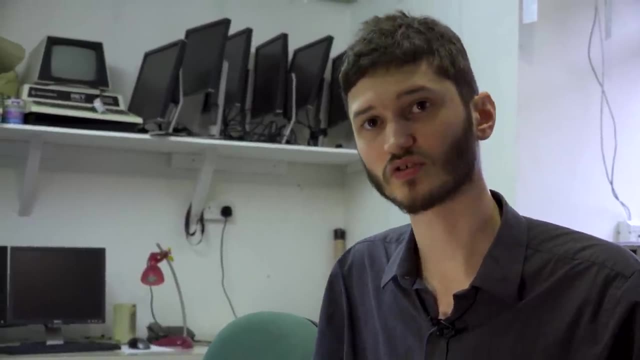 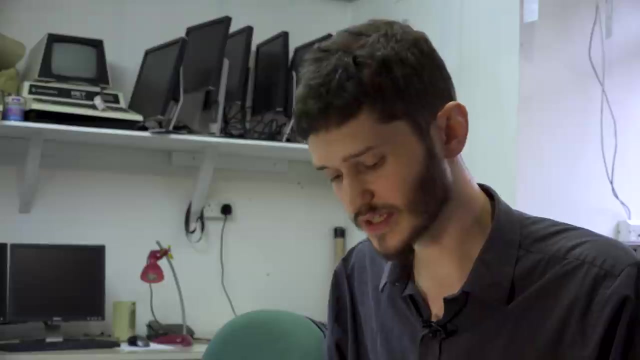 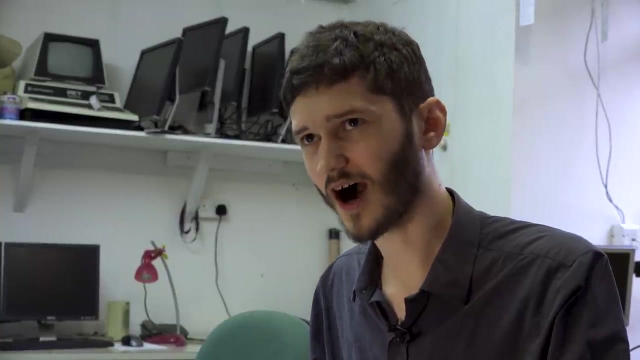 So generally you're trying to move down the gradient of error for the network, Like if you're training a thing to just recognize cats and dogs. you're just moving it down the gradient towards the correct label, Whereas in this case the generator is being moved sort of up the gradient for the discriminator's error. 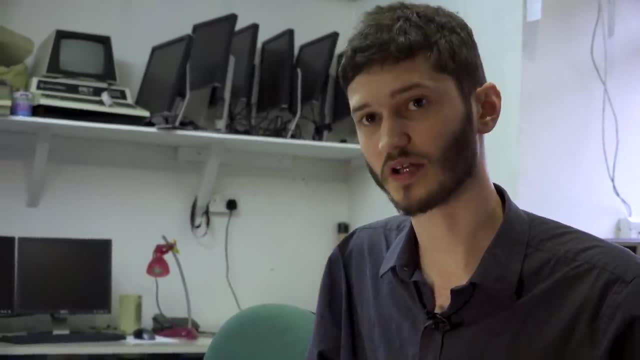 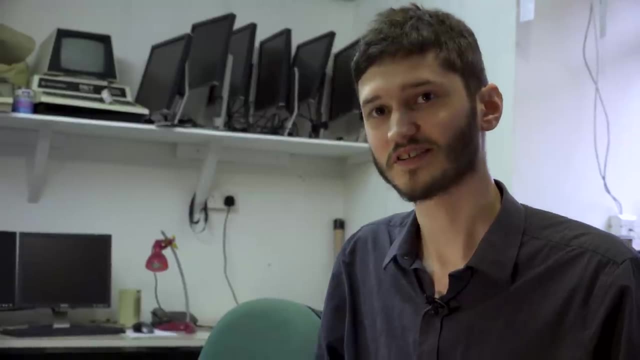 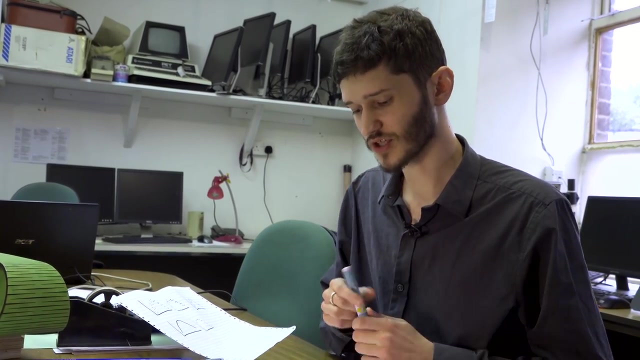 So it can find out. not just you did well or you did badly, but here's how to tweak your weights so that the discriminator would have been more wrong, so that you can confuse the discriminator more. So you can think of this whole thing. an analogy people sometimes use is like a forger. 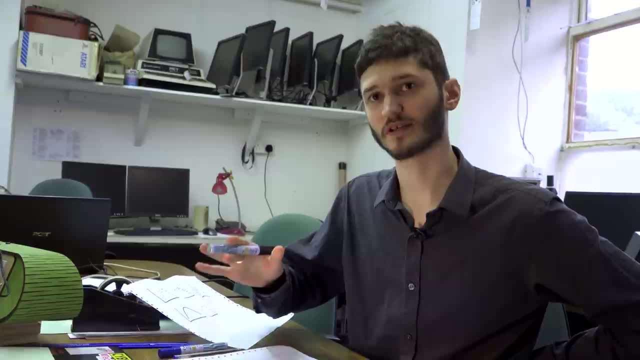 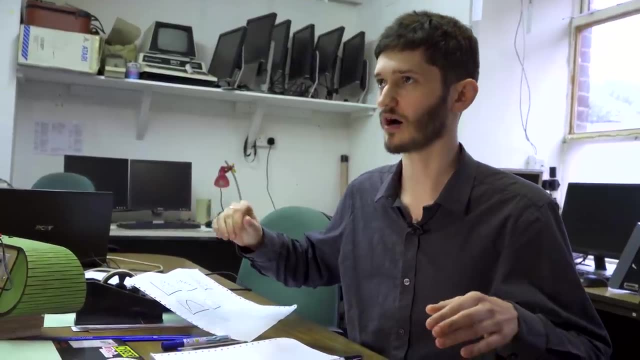 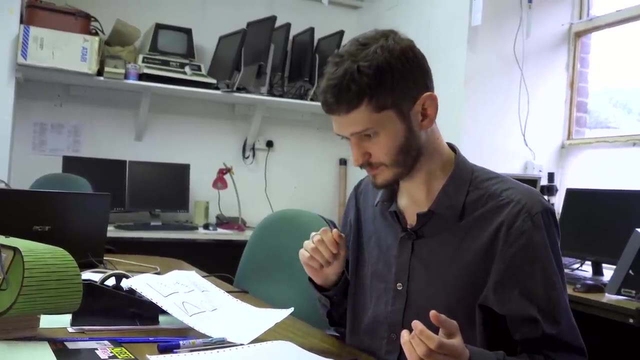 and an expert investigator person right At the beginning. let's assume there's one forger and there's one investigator and all of the art buyers of the world are idiots At the beginning. the level of the quality of the forgeries is going to be quite low, right. 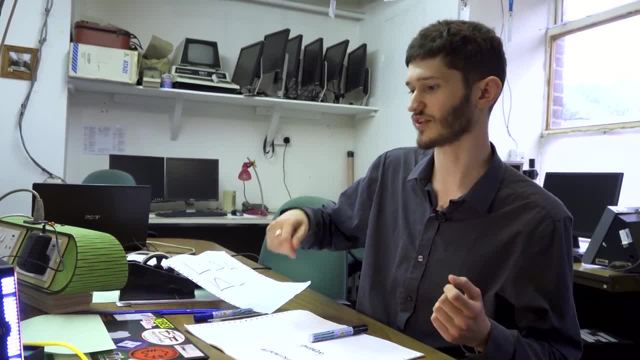 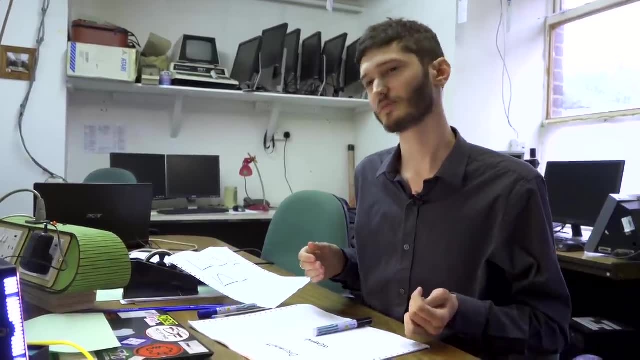 The guy just gets some paint and then he just writes, you know, Picasso on it, and he can sell it for a lot of money. And the investigator comes along and says, eh, I'm not sure, I don't think that's right. 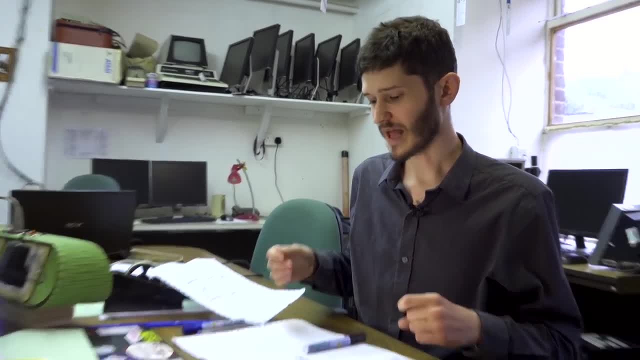 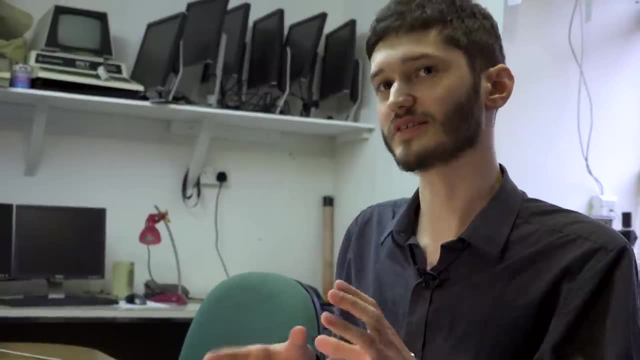 or maybe it is, I'm not sure, I haven't really figured it out. And then, as time goes on, the investigator, who is the discriminator, will start to spot certain things that are different between the things that the forger produces and real paintings. 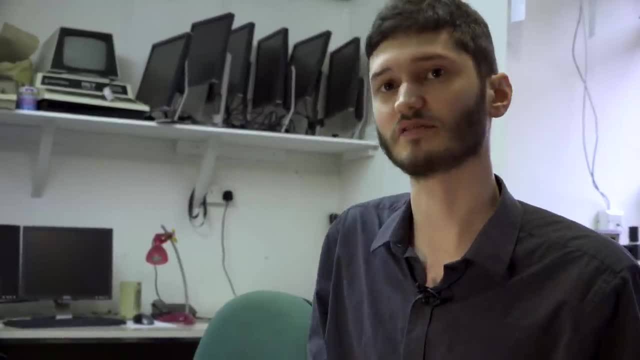 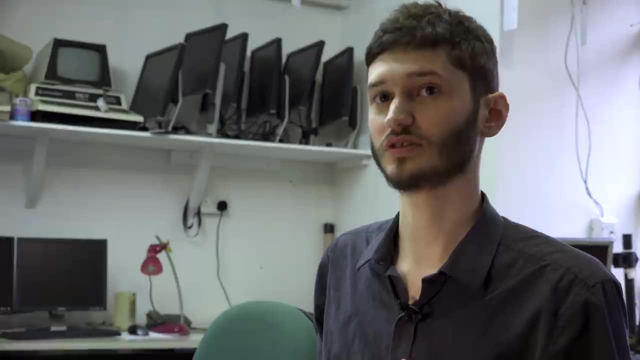 And then they'll start to be able to reliably spot. oh, this is a fake. you know this uses the wrong type of paint or whatever. so it's fake. And once that happens, the forger is forced to get better right. 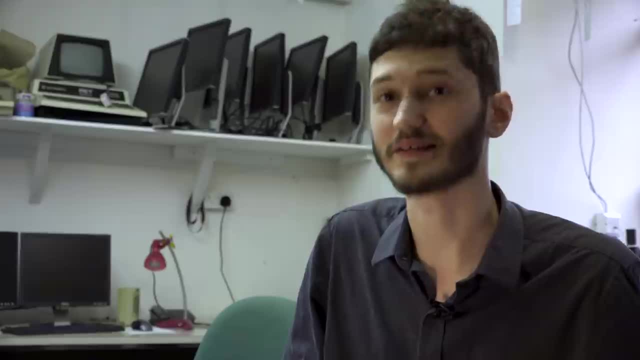 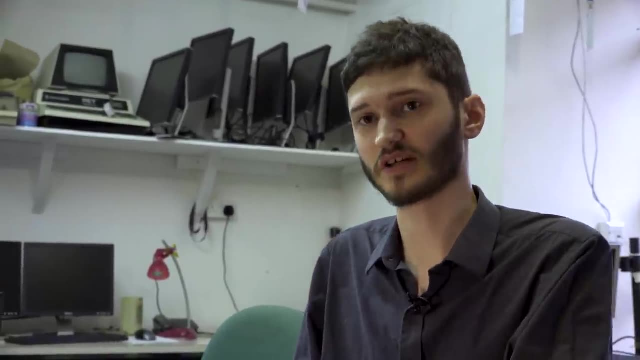 He can't sell his fakes anymore. he has to find that kind of paint. So he goes and, you know, digs up Egyptian mummies or whatever to get the legit paint, And now he can forge again. and now the discriminator, the investigator, is fooled. 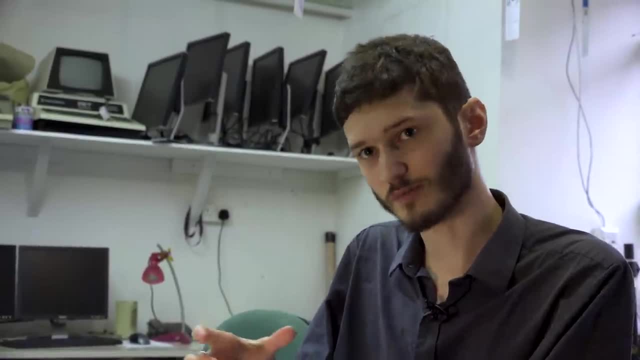 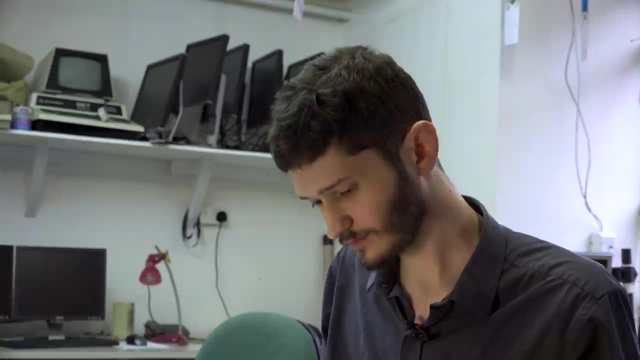 And they have to find a new thing that distinguishes the real from the fakes, And so on and so on. in a cycle they force each other to improve, And it's the same thing here. So at the beginning the generator is making just random noise, basically. 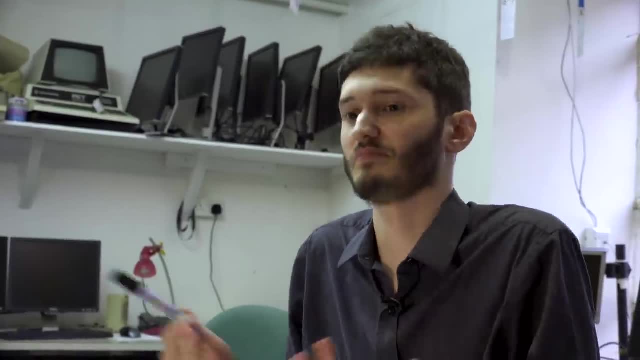 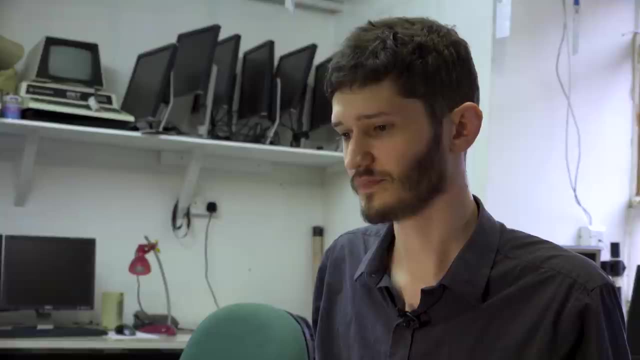 because it's getting random noise in and it's doing something to it who knows what, and it spits out an image And the discriminator goes that looks nothing like a cat. And then eventually, because the discriminator is also not very smart at the beginning, right. 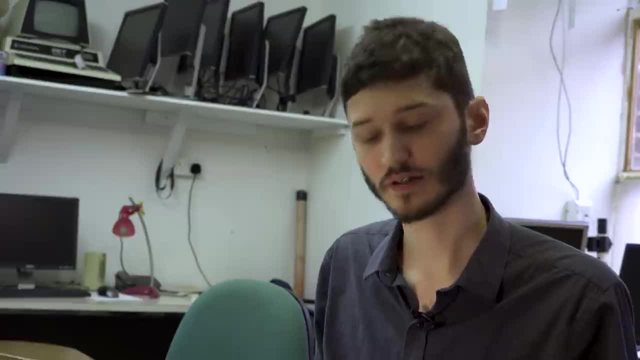 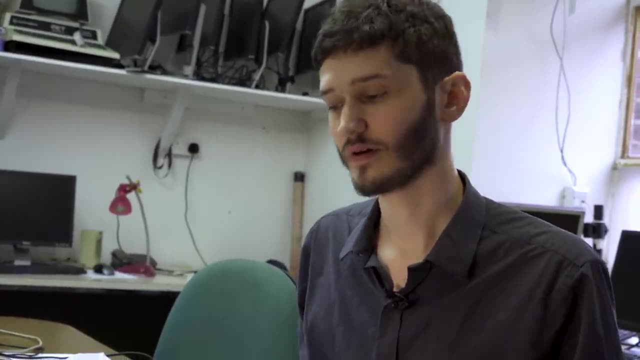 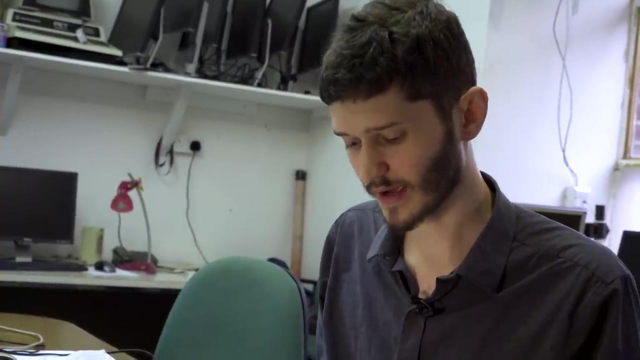 And they both get better and better. The generator gets better at producing cat-looking things and the discriminator gets better and better at identifying them, Until eventually, in principle, if you run this for long enough, theoretically, you end up with a situation where the generator is creating images. 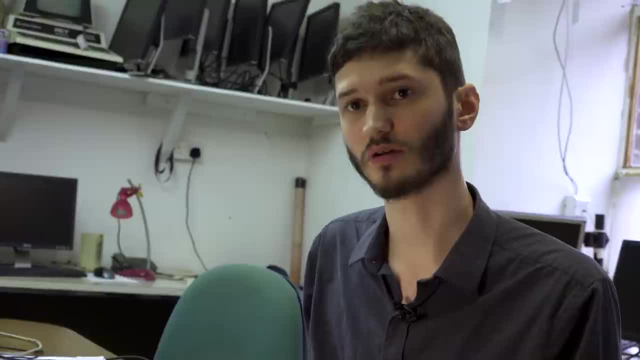 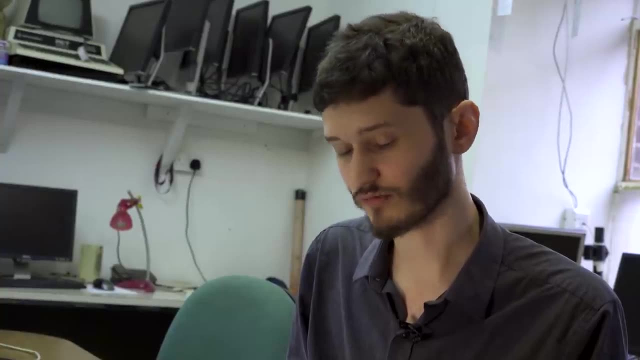 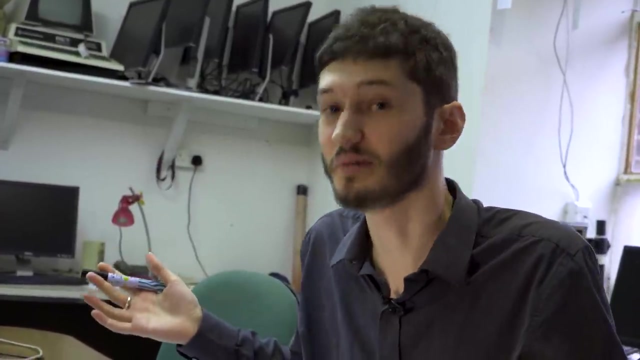 that look exactly indistinguishable from images from the real dataset And the discriminator, if it's given a real image or a fake image, always outputs 0.5.. 50-50, I don't know, Could be either. These things are literally indistinguishable. 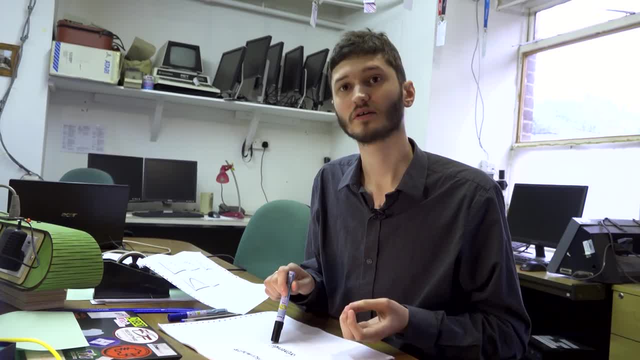 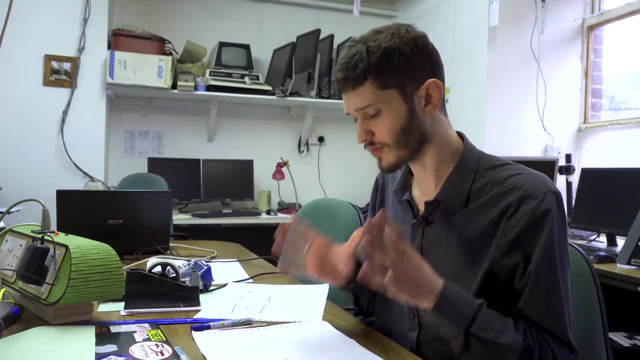 Then you pretty much can throw away the discriminator and you've got a generator which you give random noise to and it outputs brand new, indistinguishable images of cats. There's another cool thing about this, which is every time we ask the generator to generate a new image. 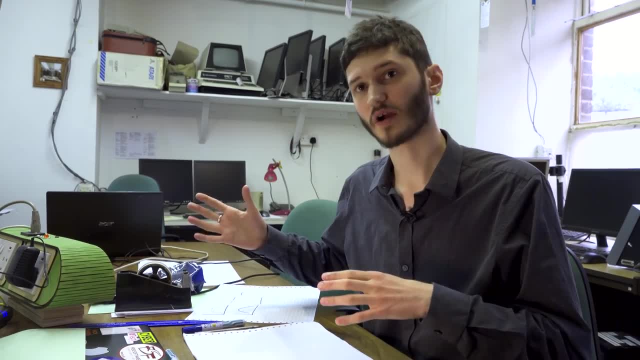 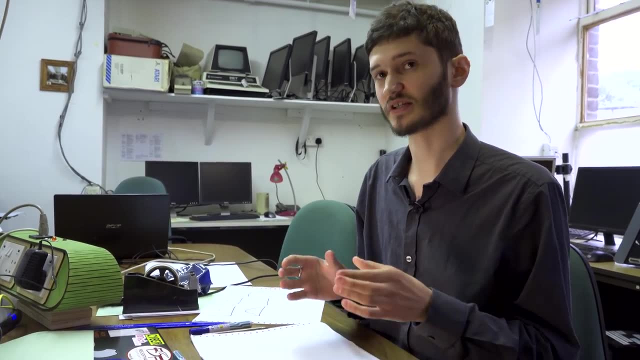 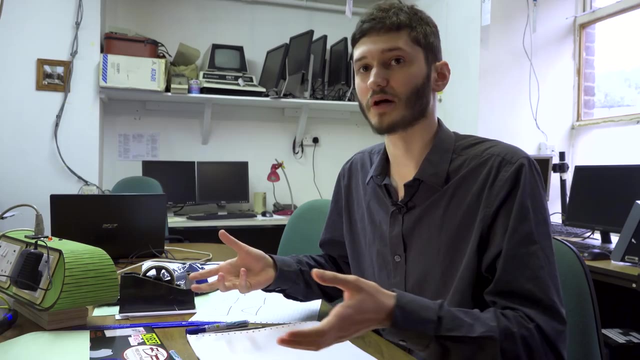 we're giving it some random data, right. We give it just this vector of random numbers, which you can think of as being a randomly selected point in a space, Because if you give it 10 random numbers between 0 and 1 or whatever, 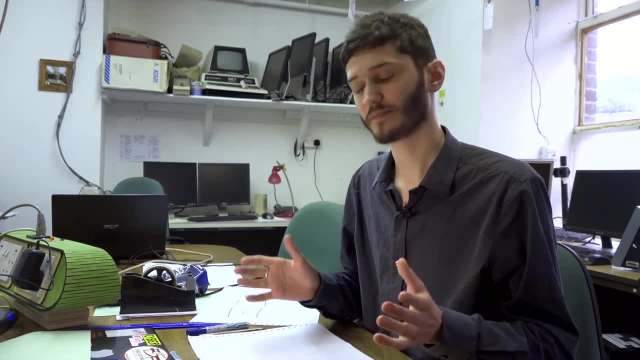 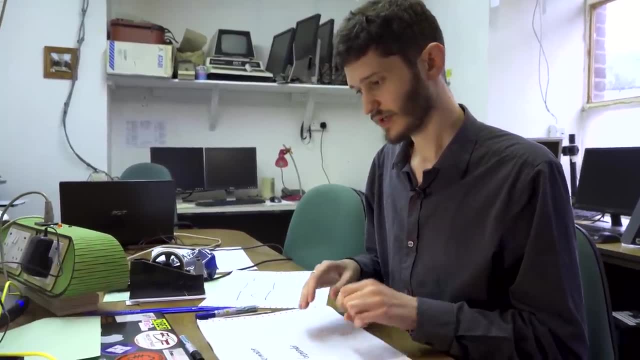 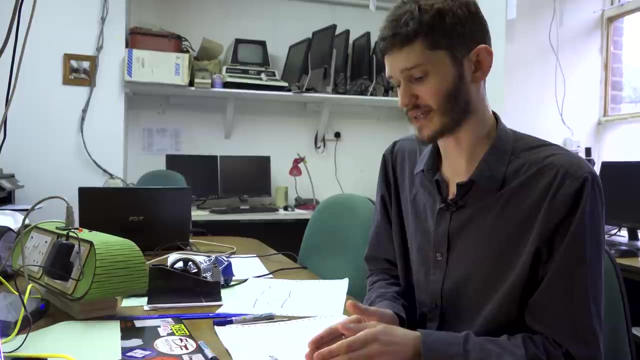 that is effectively a point in a 10-dimensional space, And the thing that's cool is that, as the generator learns, the generator is effectively making a mapping from that space into cat pictures. This is called a latent space, by the way, generally. 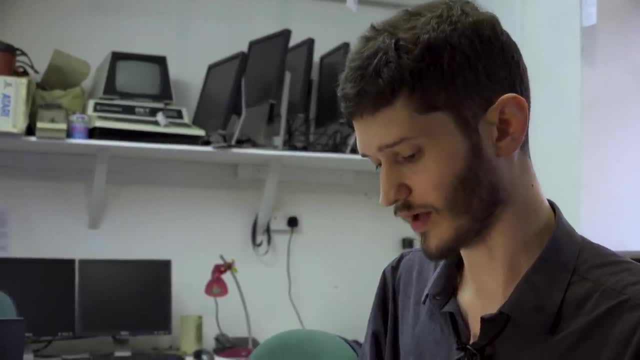 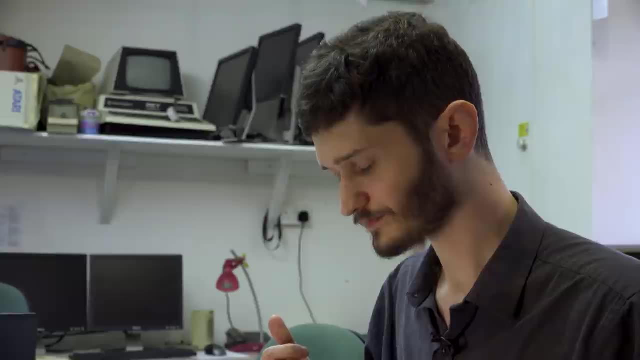 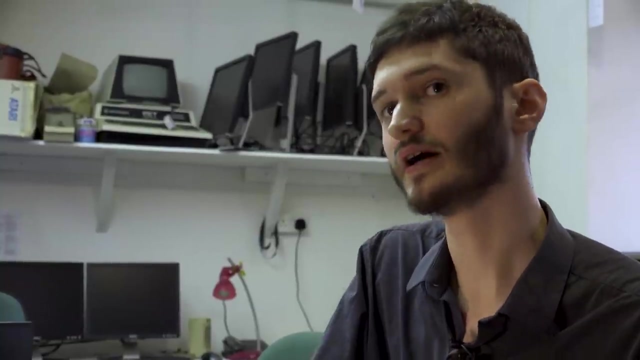 Any two nearby points in that latent space will, when you put them through the generator, produce similar cat pictures, similar pictures in general. Which means as you move around, if you take that point and smoothly move it around the latent space, you get a smoothly varying picture of a cat. 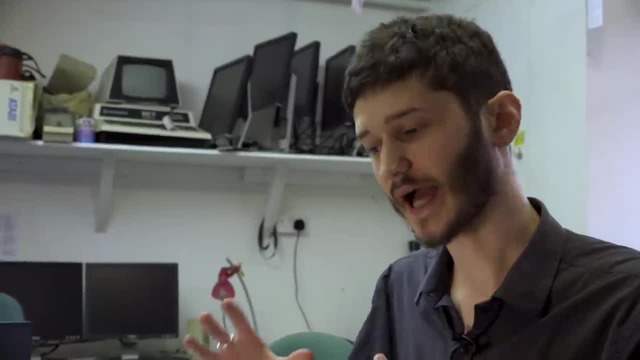 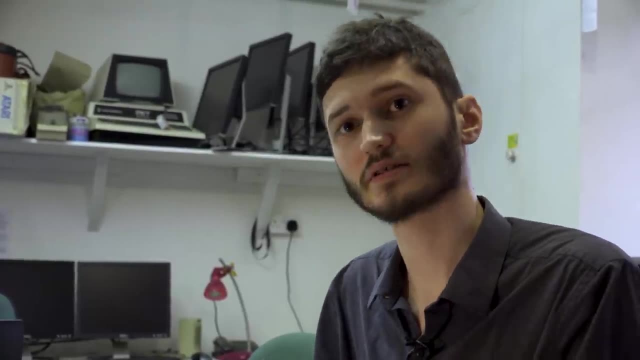 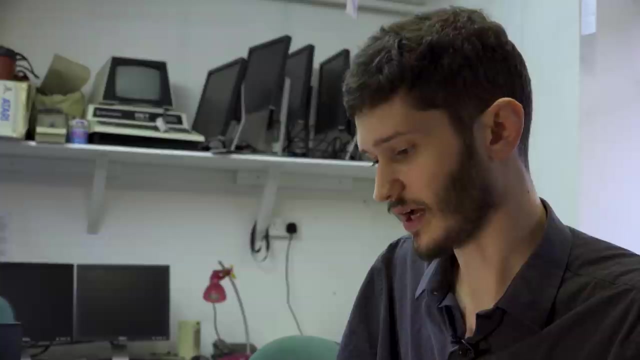 And so the directions you can move in the space actually end up corresponding to something that we as humans might consider meaningful about cats. So there's one direction and it's not necessarily one dimension of the space or whatever, and it's not necessarily linear or a straight line or anything. 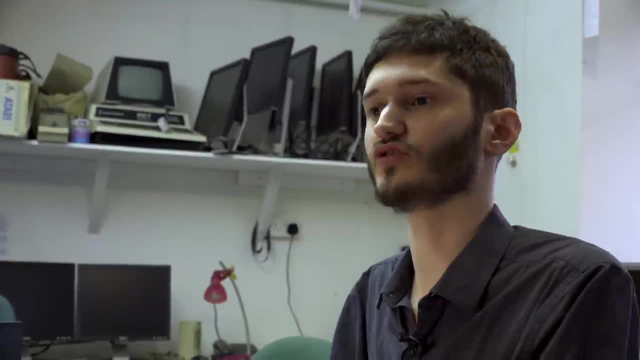 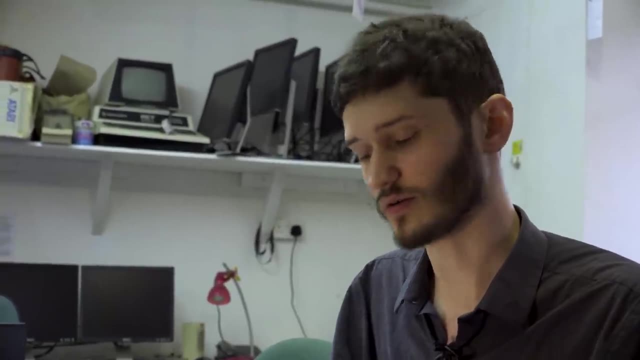 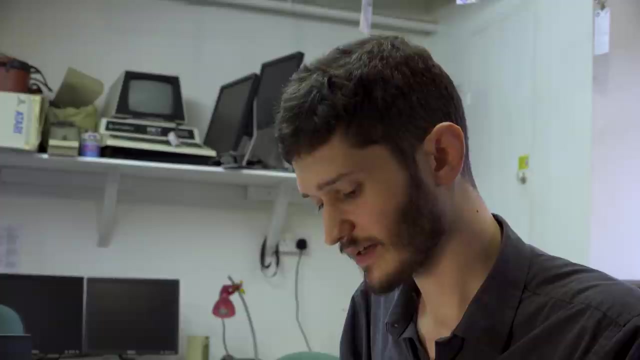 but there will be a direction in that space which corresponds to how big the cat is in the frame, for example, Or another dimension will be the color of the cat, or whatever. So that's really cool, because it means that by Intuitively, you think. 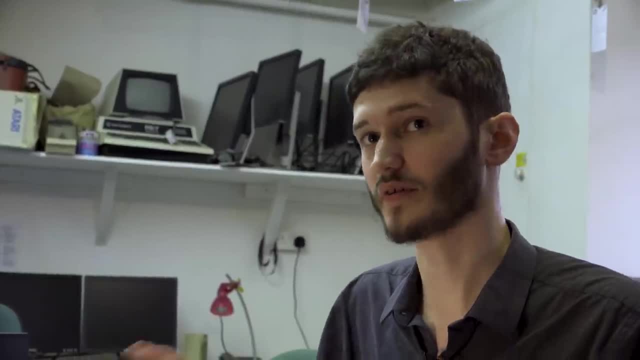 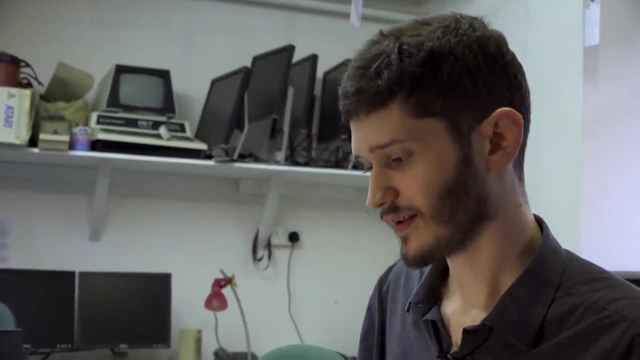 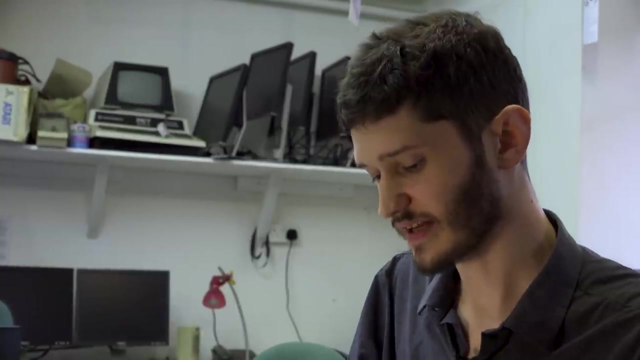 the fact that the generator can reliably produce a very large number of images of cats means it must have some understanding of what cats are, or at least what images of cats are, And it's nice to see that it has actually structured its latent space in this way. 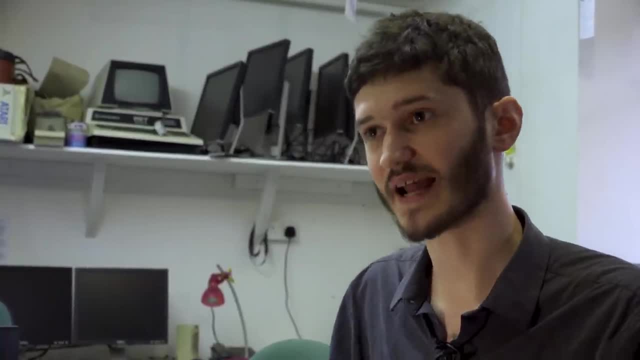 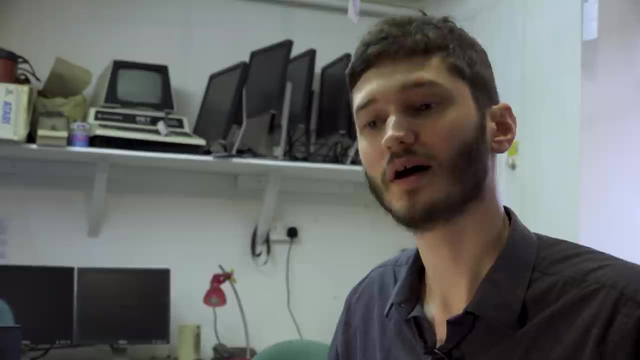 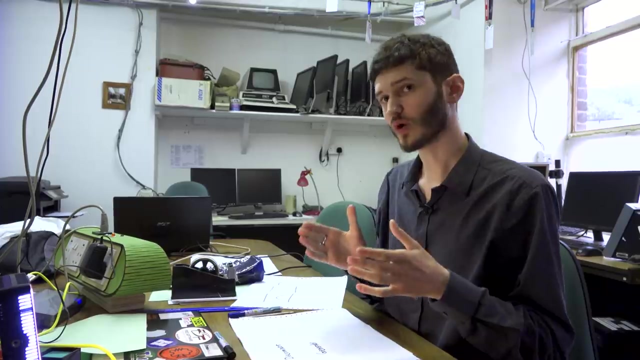 that by looking at a huge number of pictures of cats, it has actually extracted some of the structure of cat pictures in general in a way which is meaningful When you look at it, And that means you can do some really cool things. So one example was they trained one of these systems. 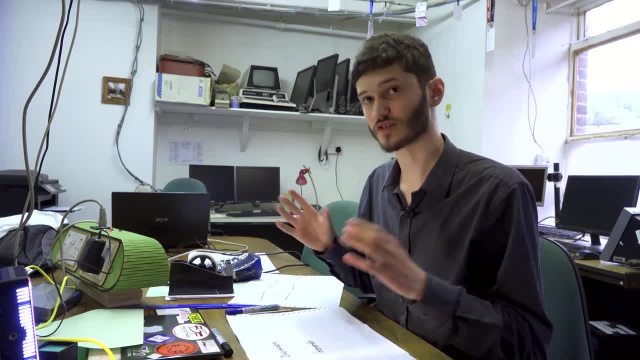 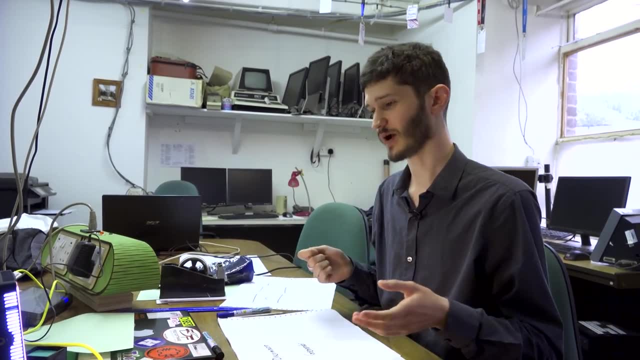 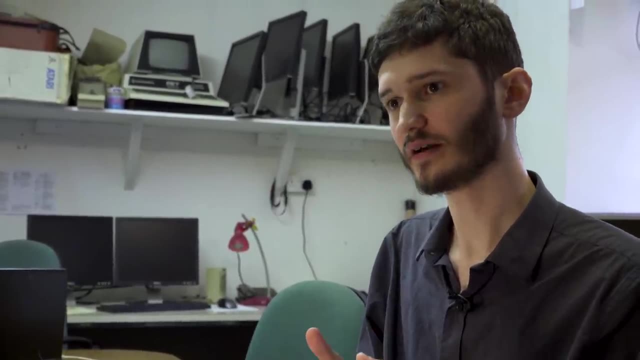 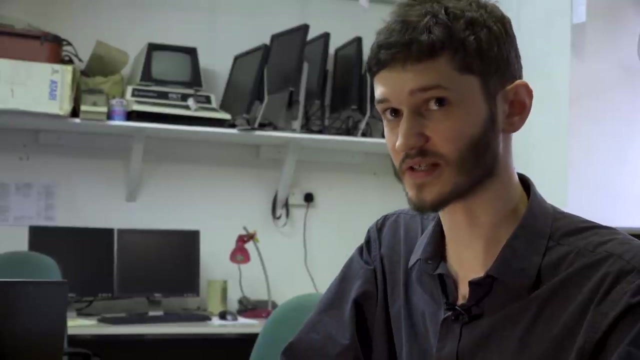 on a really large database of just face photographs, And so it could generate an arbitrarily large number of- well as large as the input space- a number of different faces. And so they found that actually, by doing basic arithmetic like just adding and subtracting vectors on the latent space, 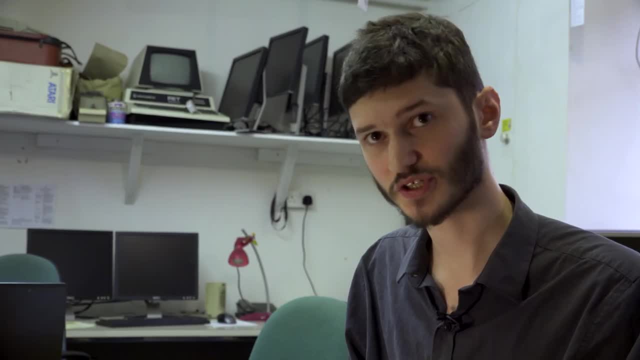 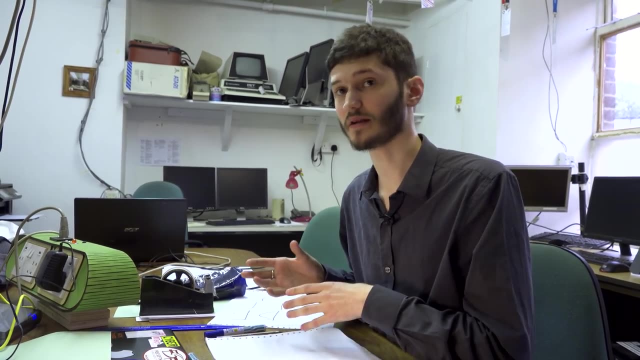 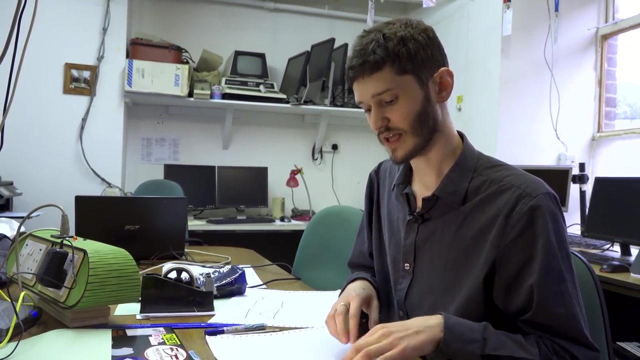 would actually produce meaningful changes in the image. If you took a bunch of latent vectors which, when you give them to the generator, produce pictures of men, and a bunch of them that produce pictures of women, and average those, you get a point in your latent space. 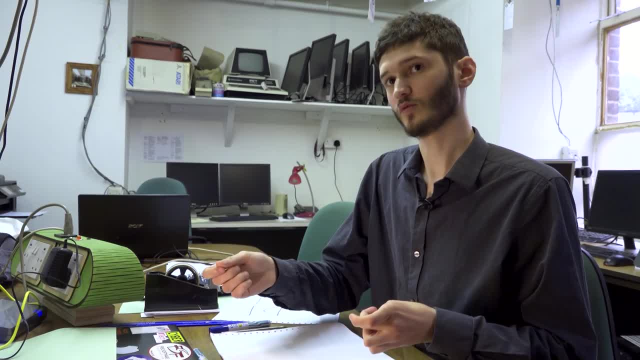 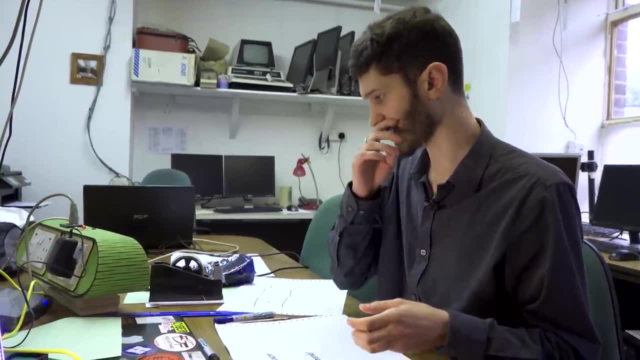 which corresponds to a picture of a man or a picture of a woman, which is not one of your inputs, It's not points, but it's sort of representative. And then you could do the same thing and say, oh, I only want give me the average point of all of the things. 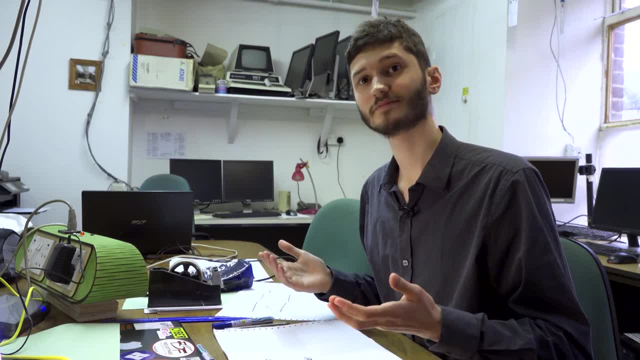 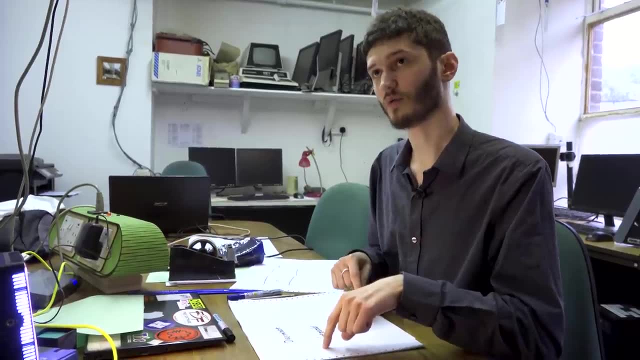 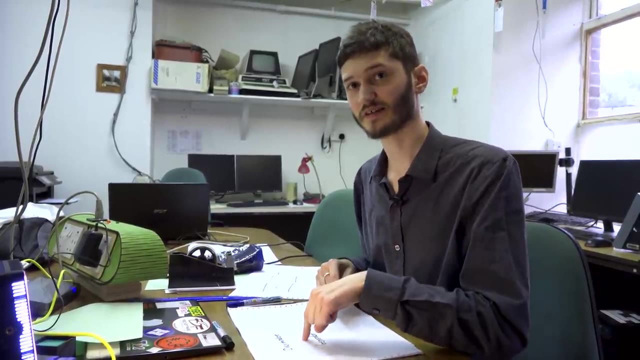 that correspond to pictures of men wearing sunglasses Right. And then if you take your sunglass vector, your men wearing sunglasses vector, subtract the man vector and add the woman vector, you get a point in your space. And if you run that through the generator, 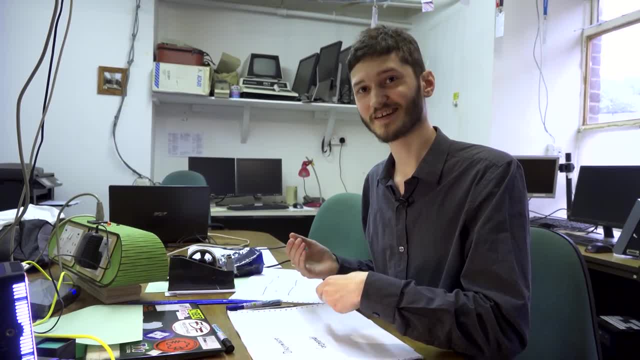 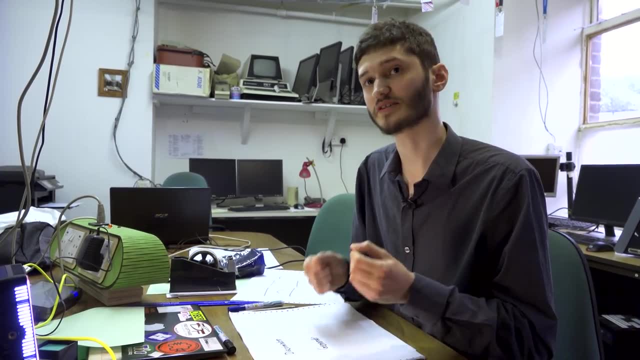 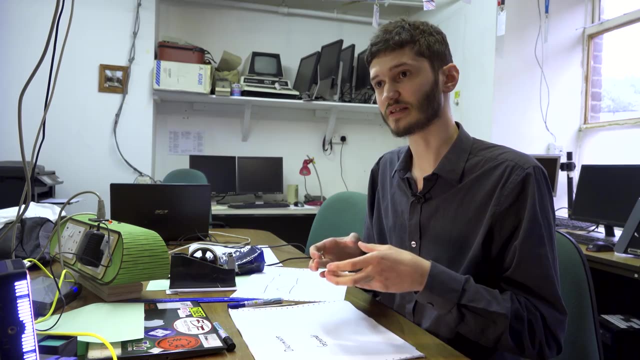 you get a woman wearing sunglasses Right, So doing basic vector arithmetic in your input space actually is meaningful in terms of images in a way that humans would recognize, which means that there's a sense in which the generator really does have an understanding of wearing sunglasses or not. 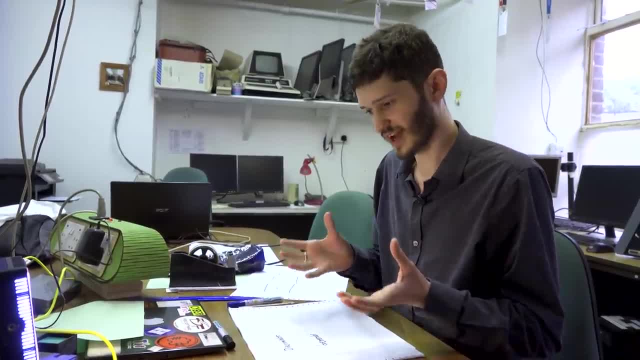 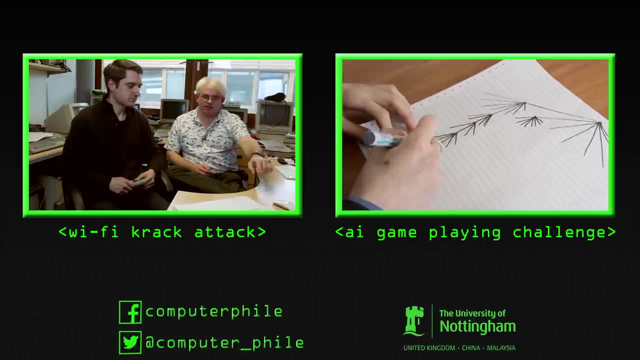 or being a man or being a woman, which is kind of an impressive result, But it's not a truly random thing, because if I know the key and I can start one and generate the same, Yeah. So I mean that, unfortunately, is the problem with cryptography.